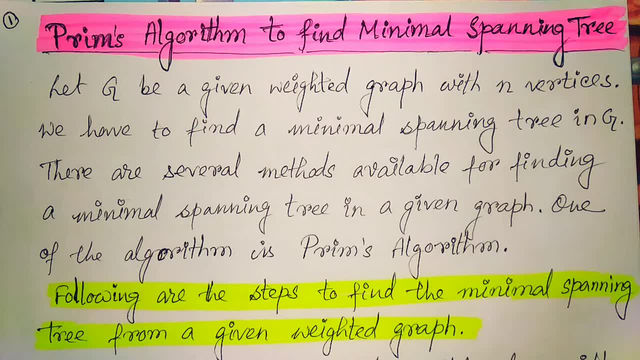 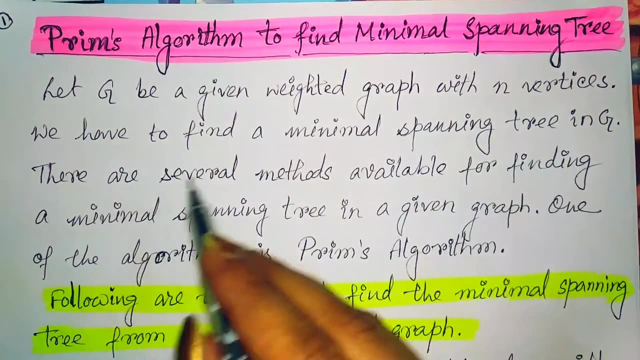 Hello friends, welcome to my YouTube channel, Easy Mathematics. In this lecture we are going to discuss the Prim's algorithm to find the minimal spanning tree. Let G be a given weighted graph with n vertices. We have to find a minimal spanning tree in G. There are several methods. 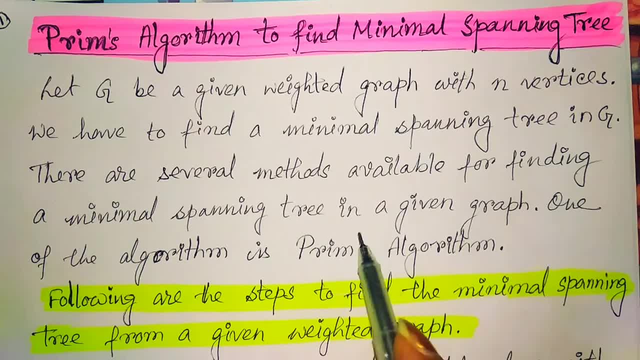 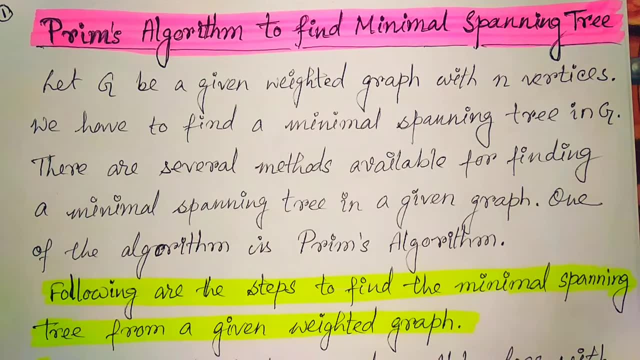 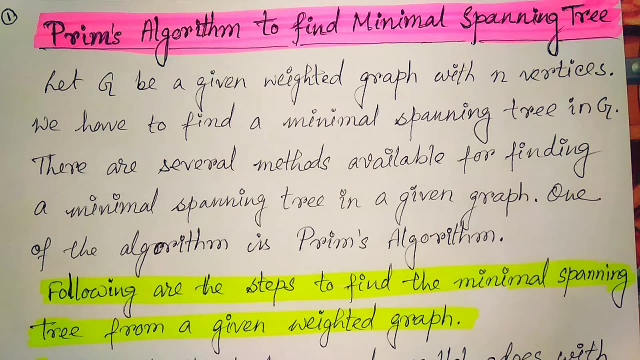 available for finding a minimal spanning tree in a given graph. One of the algorithm is Prim's algorithm. In previous lecture we have discussed one more algorithm to find out the minimal spanning tree, and that one is the Kruskal's algorithm. So now it is. 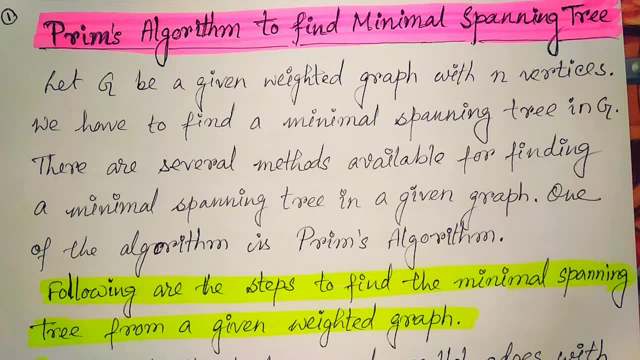 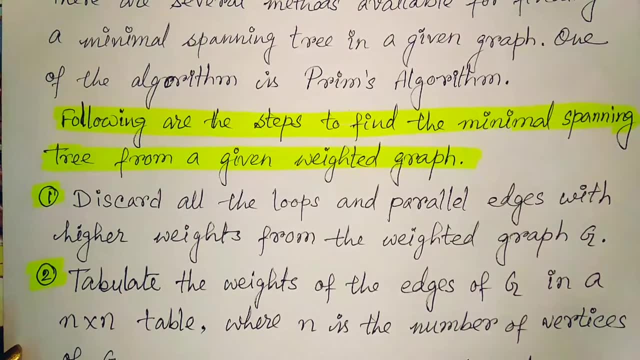 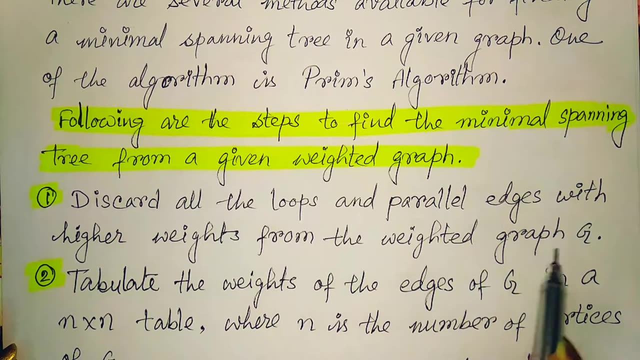 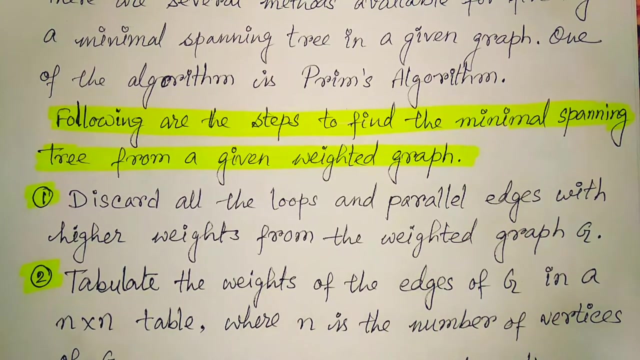 the Prim's algorithm. and here the steps: how to find out the minimal spanning tree by using the Prim's algorithm. So the first step is, as usual, it is to discard all the loops and parallel edges with higher weights from them. This is the weighted graph G. Next tabulate the weights of the edges of G in a, n, x, n table. 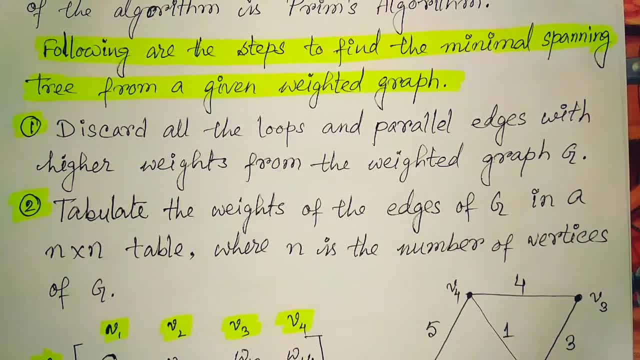 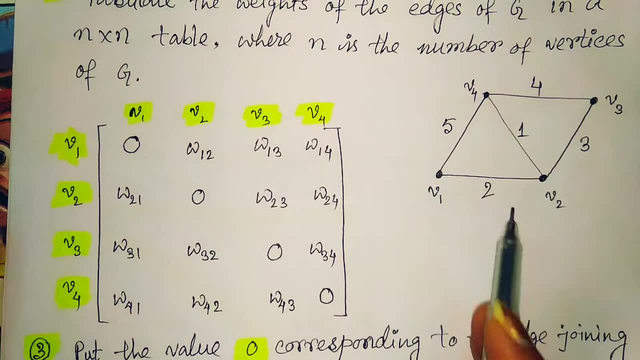 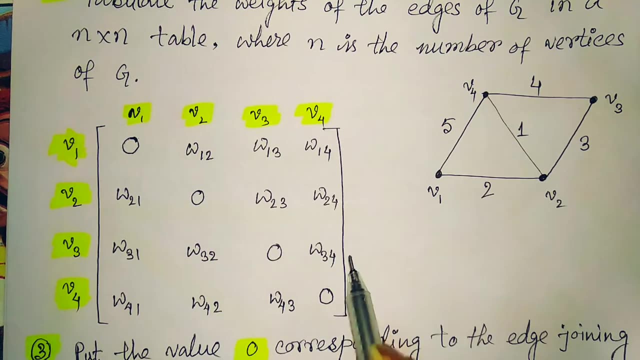 where n is the number of vertices of G. So what does it mean? Let this one is the given graph. Here the total four number of vertices are given: v1, v2, v3 and v4.. These four vertices width. we create a table where rho is equal to the number of vertices of the given graph. 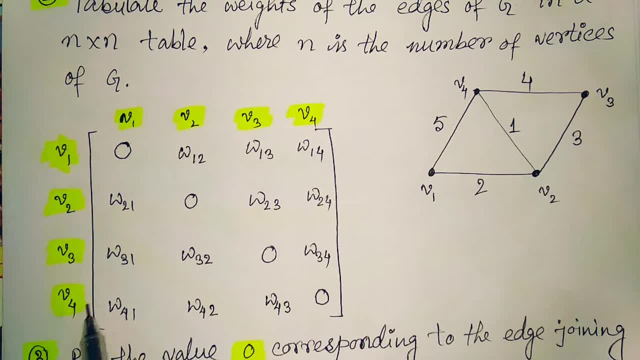 Let. this one is the given graph. Here the total four number of vertices are given: v1,, v2, v3, v4.. These all vertices and column wise also, we put the vertices v1,, v2, v3 and. 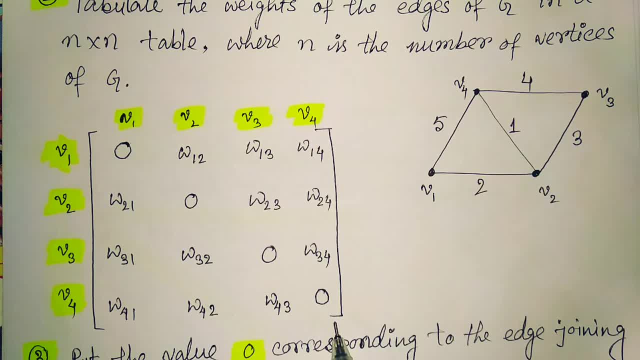 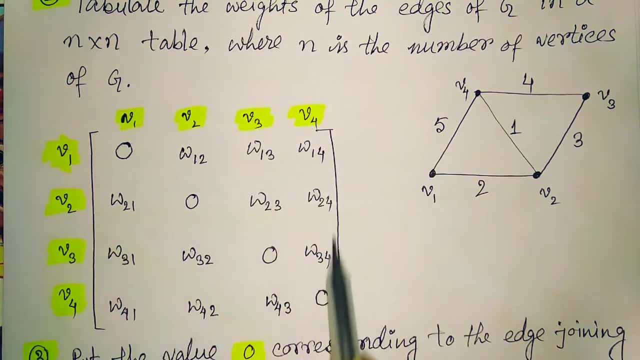 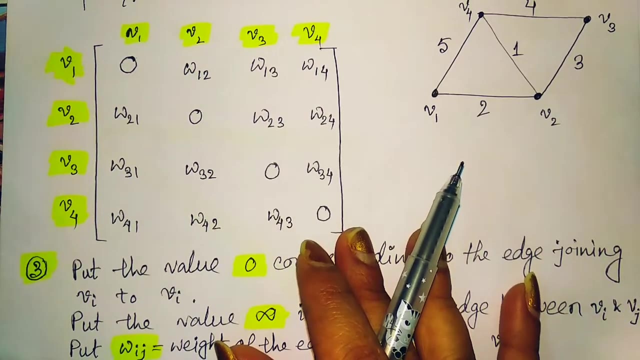 v4.. Basically, this one creates creating a four cross, four matrix. So at first, depending upon the number of vertices, we should create such matrix. After that, what about the entries of this matrix? For that we should put the value zero corresponding to this matrix. So 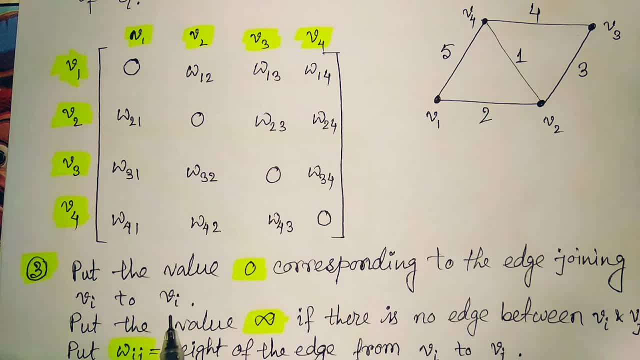 after that we start creating such matrix. So what does this mean? V1 is to the edge joining the vertex vi to vi. Vi to vi means v1 to v1, v2 to v2, v3 to v3, v4 to v4.. That means v1. 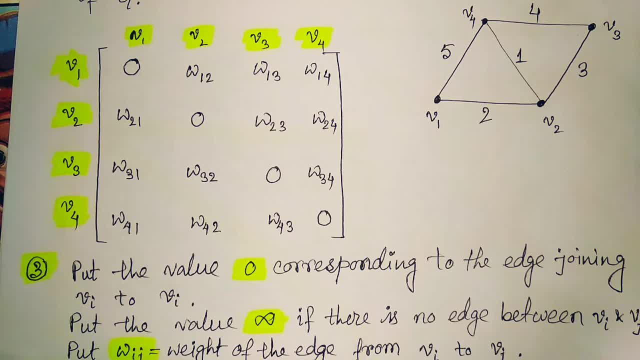 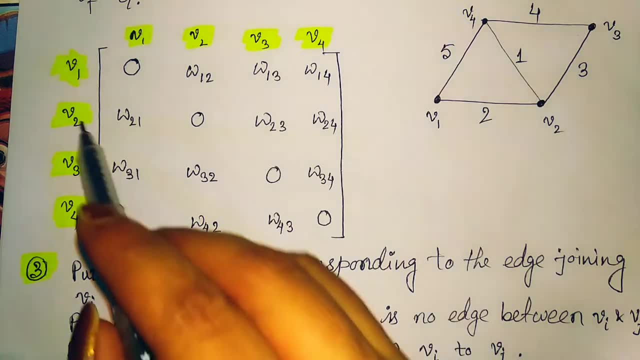 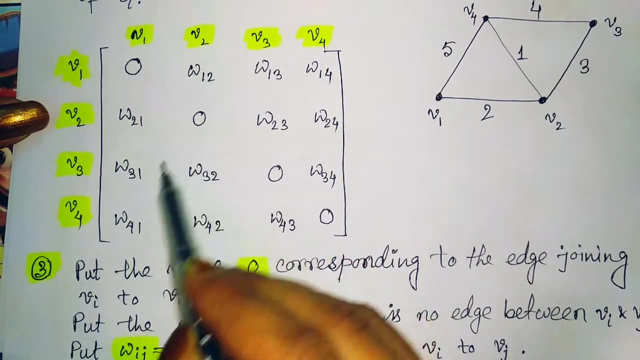 to v1. joining means there exist a loop, But in the graph we initially discard all the self loops. So if this entries, we will find out here: v1 to v1 is this position, then v2 to v2 means this position, v3 to v3 means this position and v4 to v4 means this position. 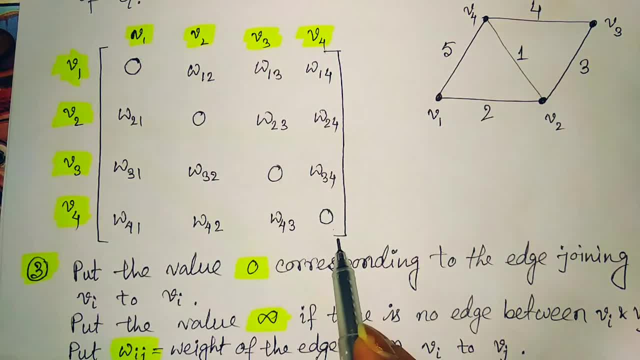 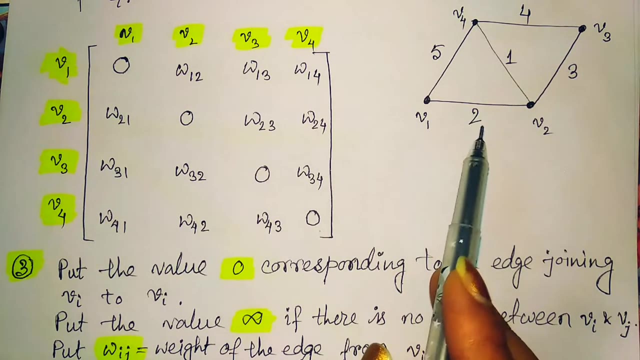 to V4 means this position. So, corresponding to all those diagonal entries, we should put the value 0.. Next put the value infinity if there is no edge between any two vertex, VI and VJ- From the given graph. if you will find out that in between two vertices there, 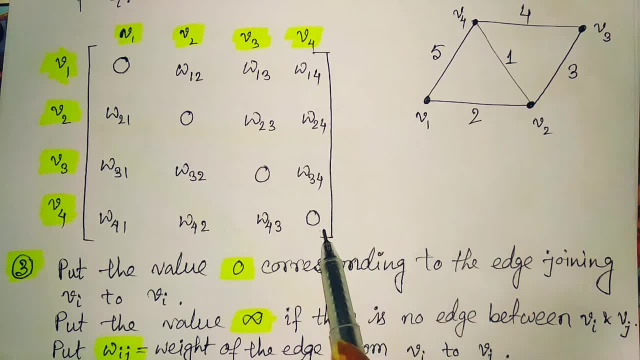 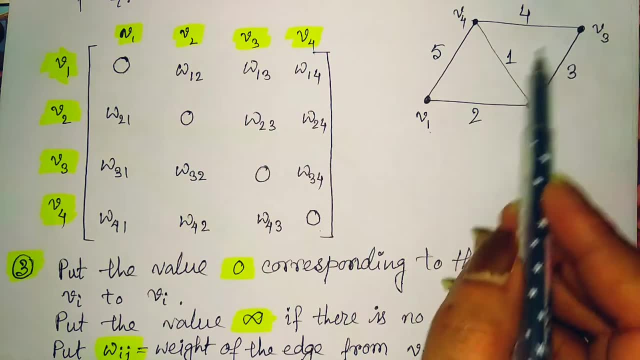 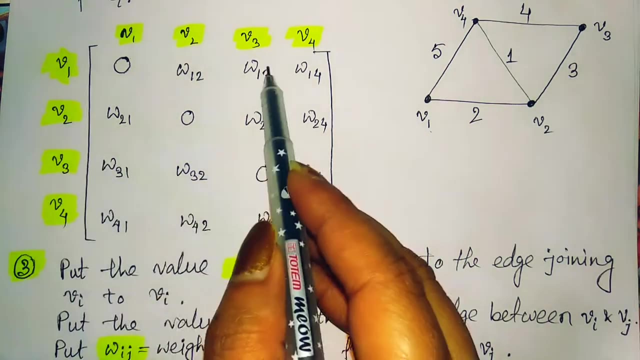 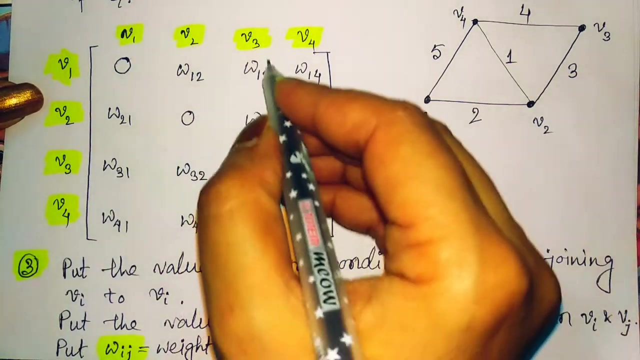 is no edge connectivity, then corresponding to that position, we should substitute the value infinity. For example, here it is V1 to V3.. These two vertices are not connected by any edge, So V1 here and V3 is here, So V1 and V3 corresponding to this one, So V1. 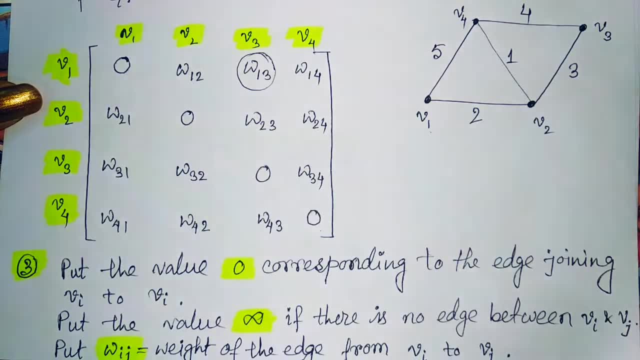 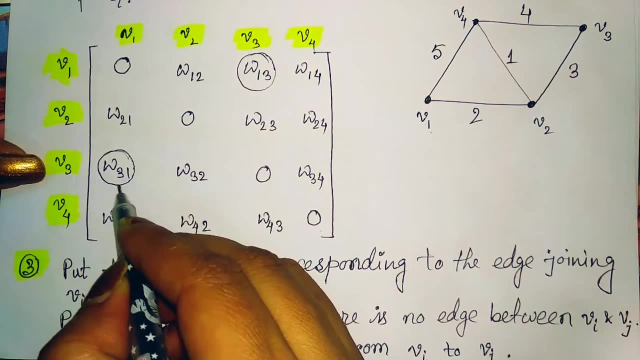 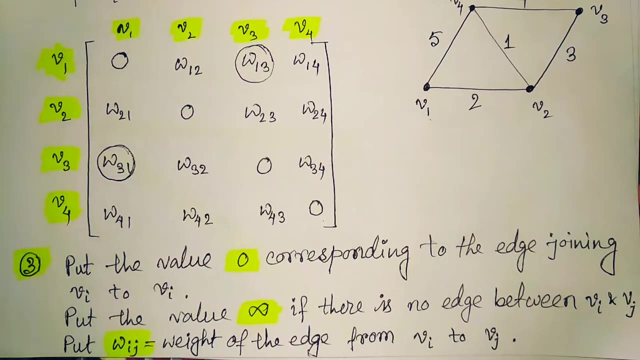 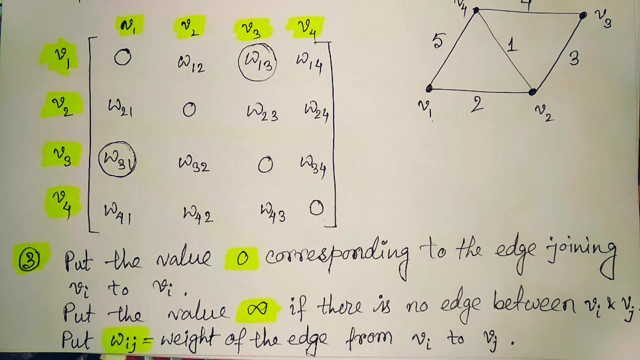 V3. that means this position should be entered as the value infinity. Similarly, V3 to V1 also put the value as infinity Because these are having the no edge connectivity. Now if in between the two different vertices there is an edge connectivity, then we should put the given weight corresponding to the 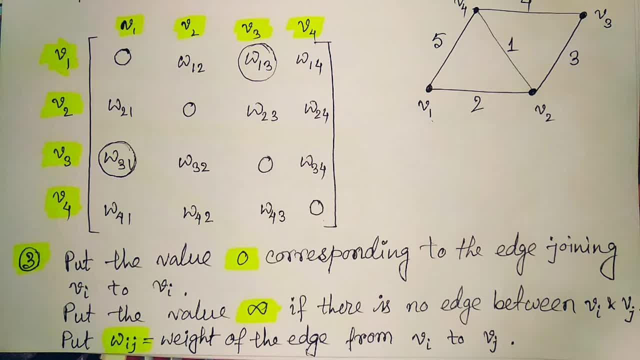 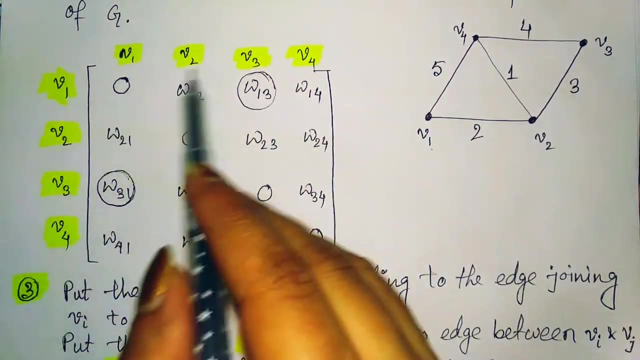 given edge. So that edge we should denote it by WIJ WIJ. in general we put the weight depending upon the vertices chosen. So here, if we consider the first row, then we just look: V1 to V2, V1 to V1, it is 0, then V1 to V2, V1 to V2, there is an edge connectivity. 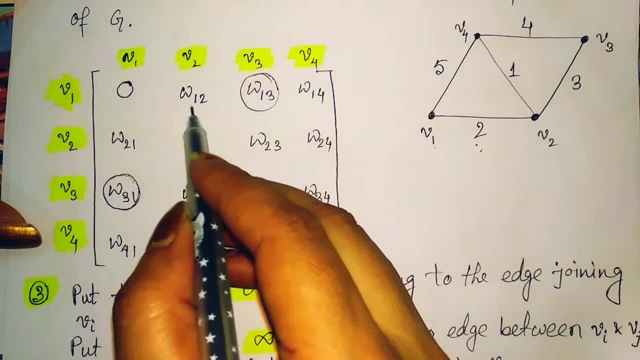 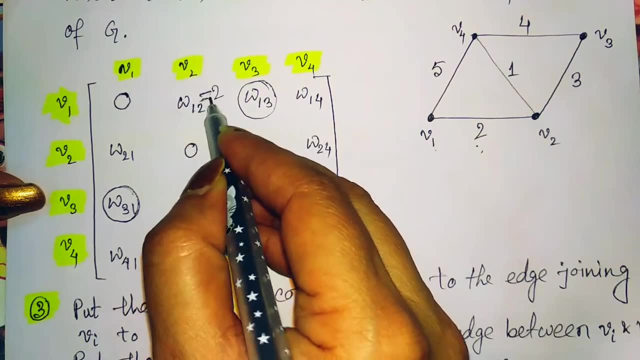 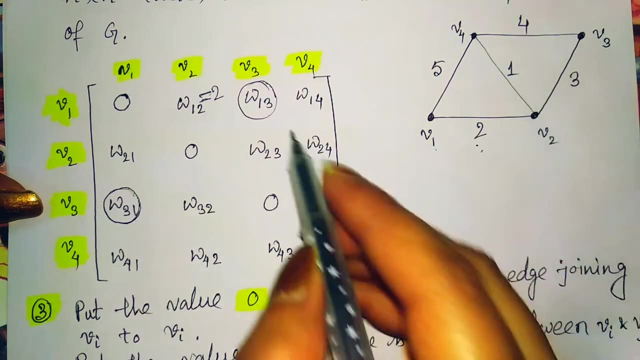 and its weight is 2.. That means W12 is the corresponding general weight and its value is equals to 2 for this particular given graph. Now, V1 to V3. as V1 to V3 no edge connectivity, then this value should be infinity. And V1 to V4, V1 to V5, V3 to V6, V1 to V7, the value. 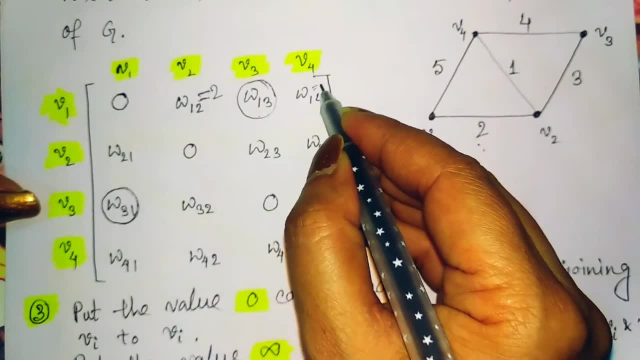 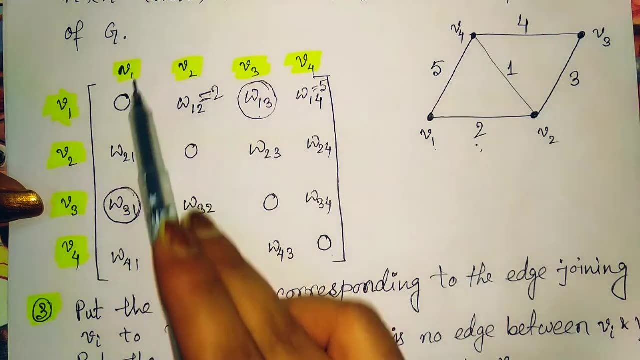 should be infinity. V1 to V4: again it is connected and this value is equals to 5, because the given weight is 5.. Similarly, now come to the vertex V2.. So V2 to V1, V2 to V1: it is connected and its value is 2.. 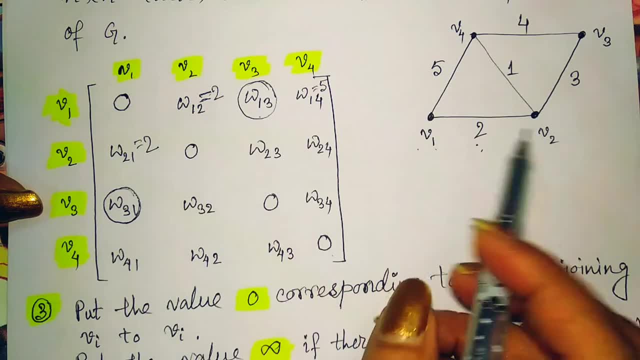 So it has to be 2.. Then V2 to V2 should be 0. Then V2 to V3, V2 to V3: it is connected and its value is 3. So that we put this value as 3.. 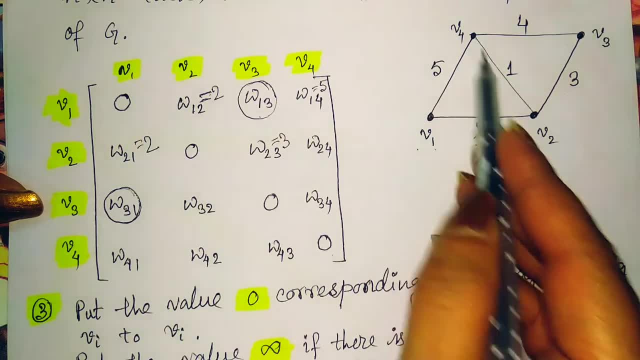 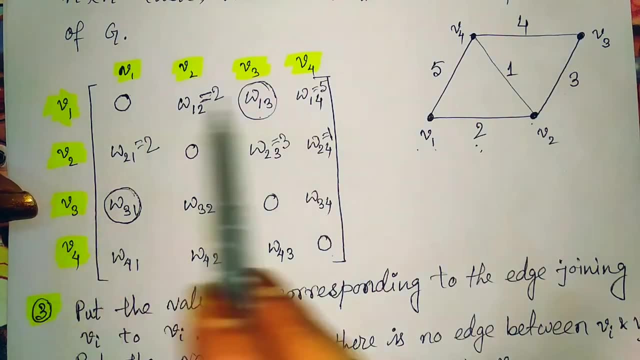 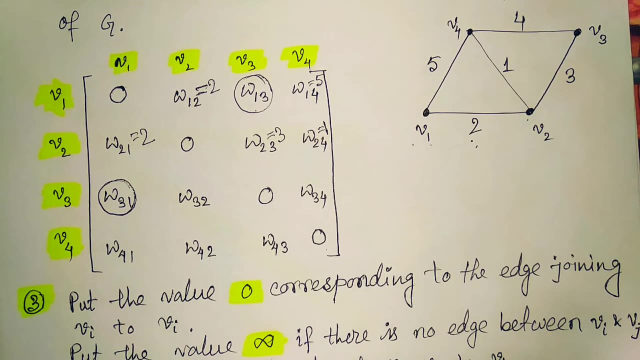 Now V2 to V4.. So, V2 to V4, the connectivity is there and its weight value is 1.. Hence this value should be 1.. And likewise we just find out the corresponding spaces where we should put the corresponding weight, depending upon the connectivity of the vertices. 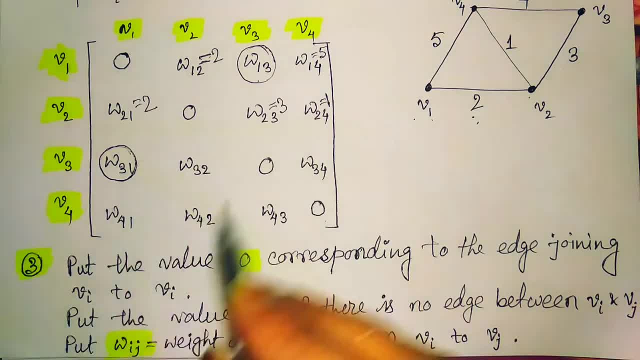 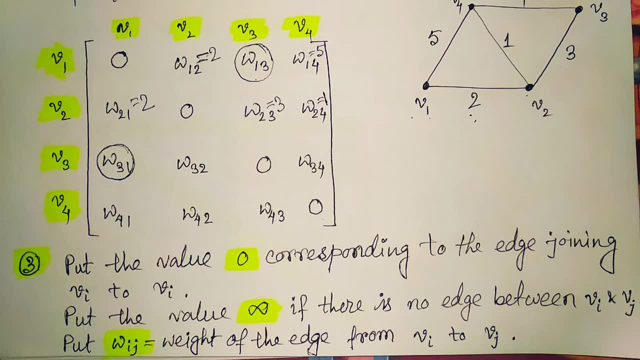 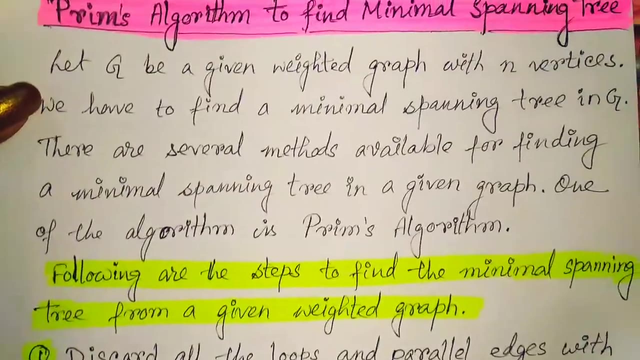 So in this way, we should make a table from which we calculate the minimal spanning tree. So this table is very much important to create. So at first We should create this table for the simple graph. Now, after creating this table, 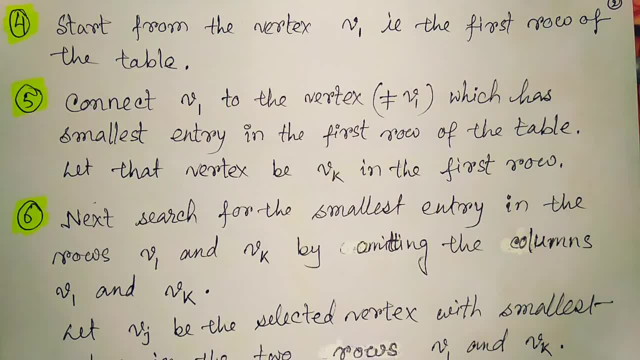 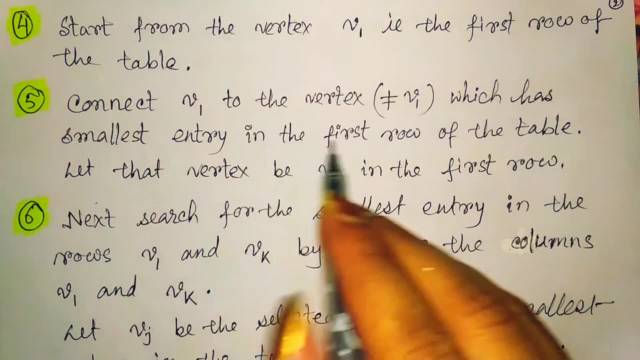 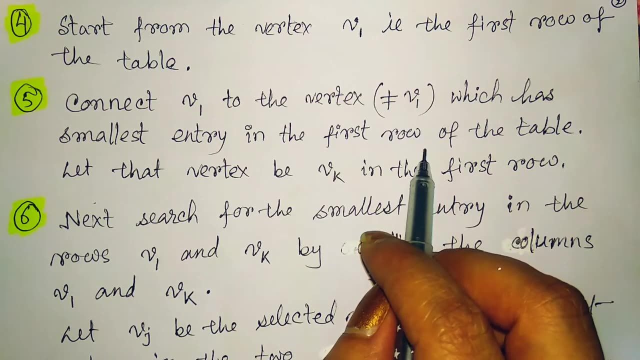 We should start from the vertex V1.. V1: that means it is the first row of the table. Now what we will do? We connect this V1 to the vertex which has smallest entry in the first row of the table. So we just observe the entire first row of the previous table. 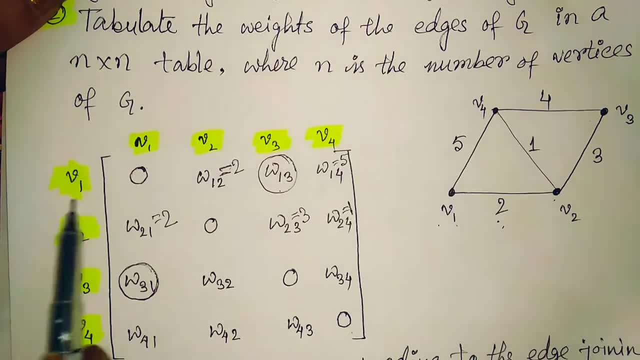 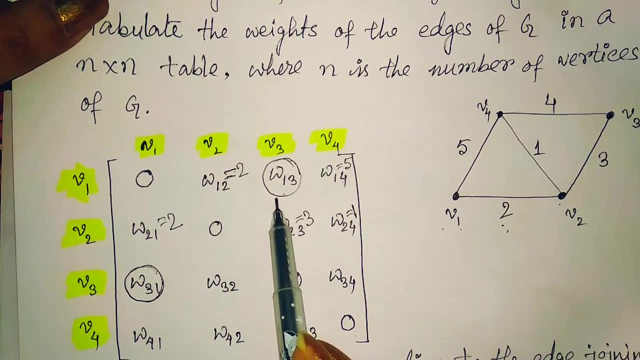 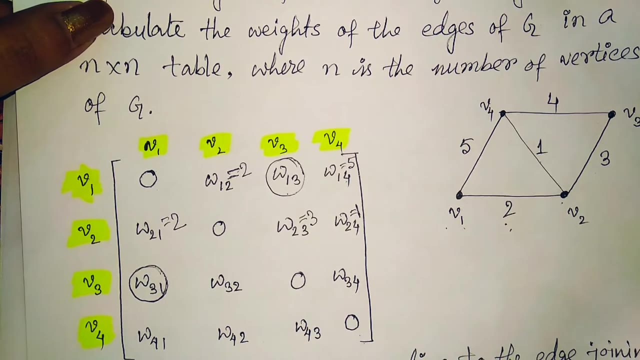 In this table we should observe the entire first row. Among this all first row entries, which value is the smallest value? Definitely 0. we should not consider, because these are the diagonal entries and infinity is the any value, So we should not consider infinity also. 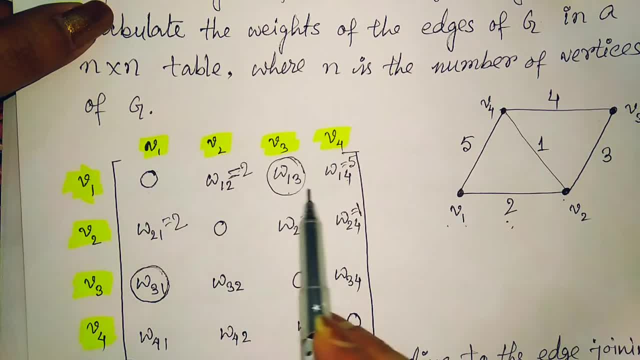 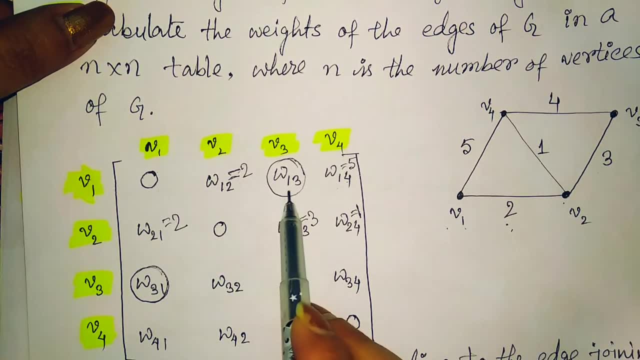 So any value if it is given, then we should consider which one is the minimum. If we consider this one, the first row, then its first entry is 0.. Second entry is 2.. Third entry is infinity and fourth entry is 5.. 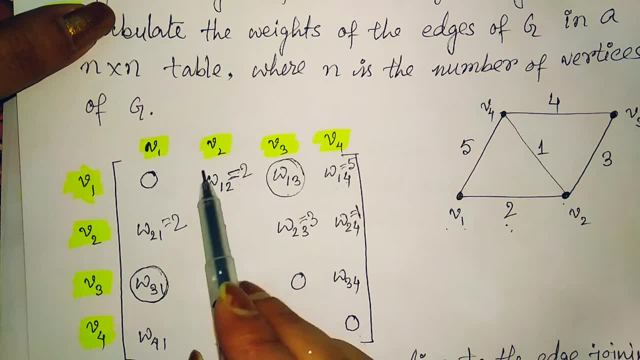 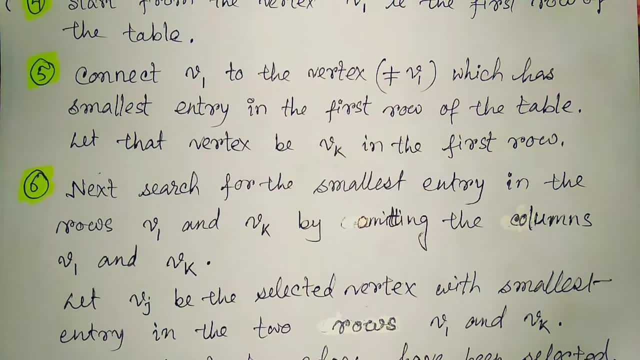 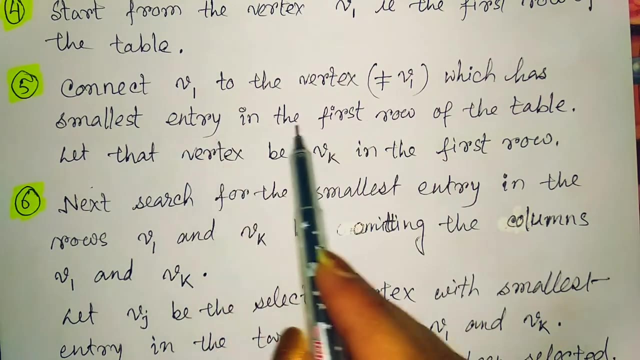 So the minimum value is 2.. That's why we should select this position, and this position is the connectivity with V1 to V2.. So what we will do here? We connect V1 to the vertex which has smallest entry in the first row of the table. 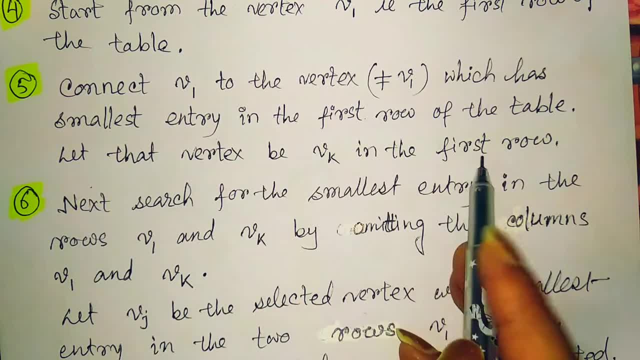 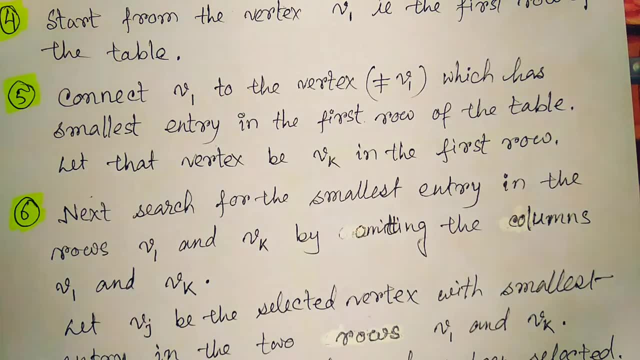 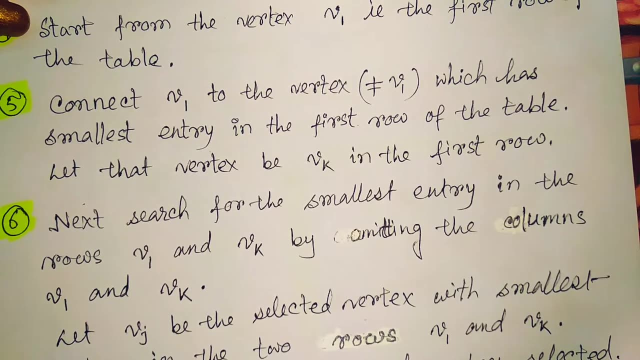 Then let that vertex be Vk in the first row. That is in general. Generally, let us consider The vertices are from V1 to Vn. Among these all vertices, we have considered that in the first row corresponding to the vertex Vk, V1, Vk. 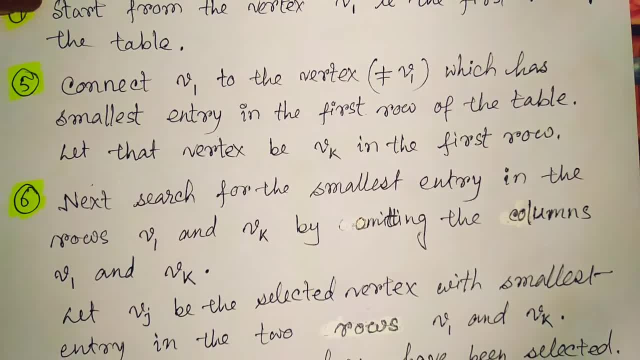 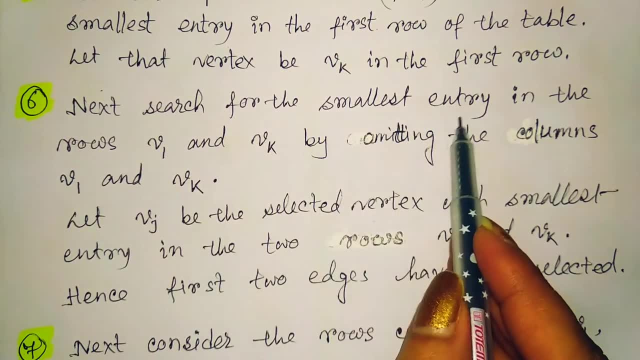 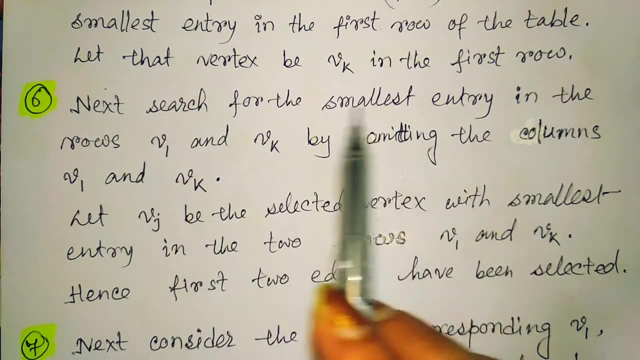 This particular entry having the minimum weight value, So we should select that one. In the next step, we should search for the smallest entry in the rows V1 and Vk Once we have started from V1 and we selected the Vk, Vk corresponding the vertex Vk. 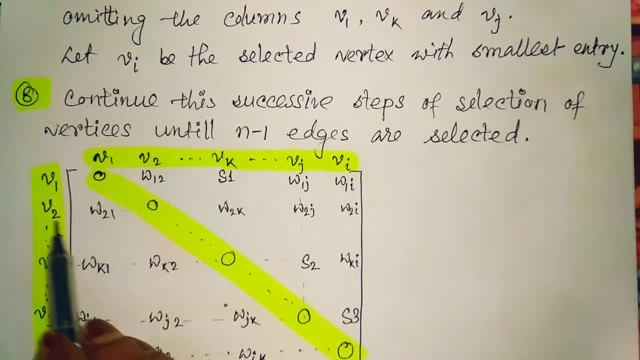 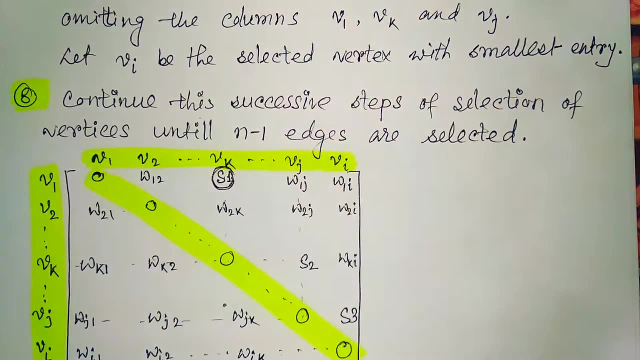 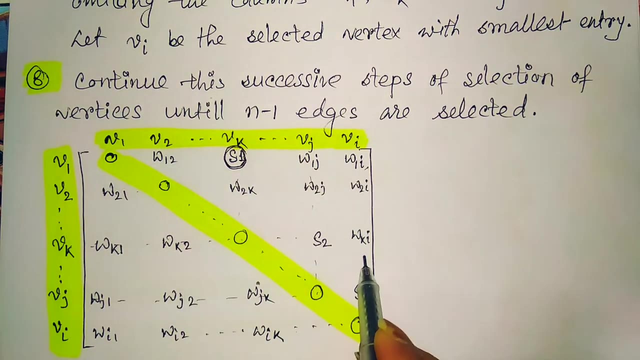 Just look, here We have started from V1.. Then let corresponding to Vk we will get. this one is the smallest entry, So that here Vk is also one of the row. So V1 is one of the row and Vk is the another row. 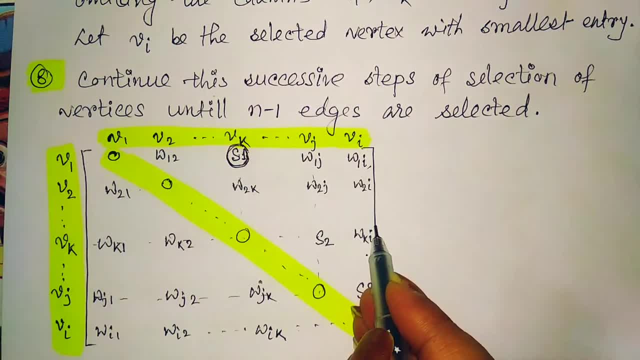 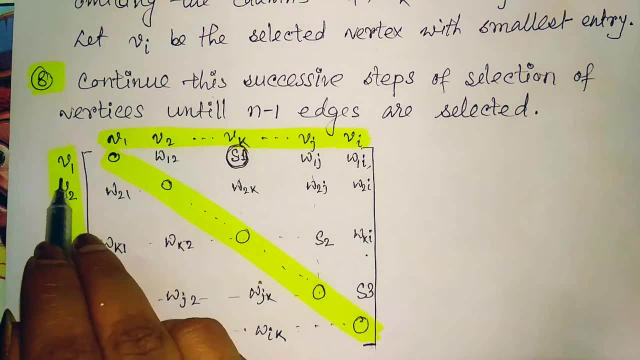 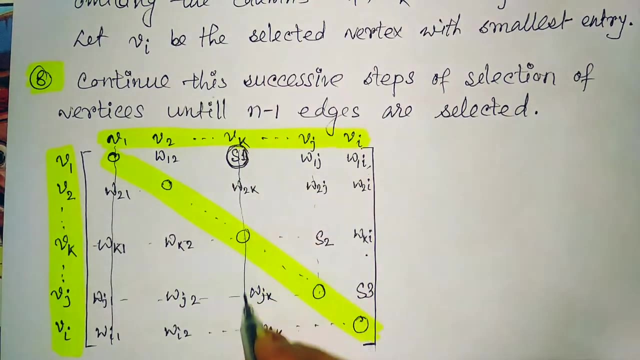 Definitely So. among these two rows we should find out the next smallest entry. But remember here, While we choose the smallest entry in V1 and Vk, That time we should not choose any of this column and this column, Because V1 and Vk- these two vertices- already has been selected. 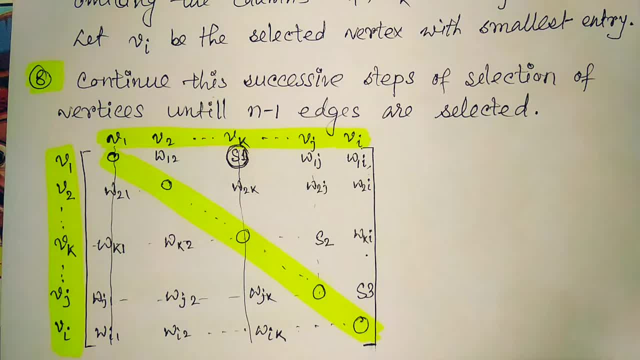 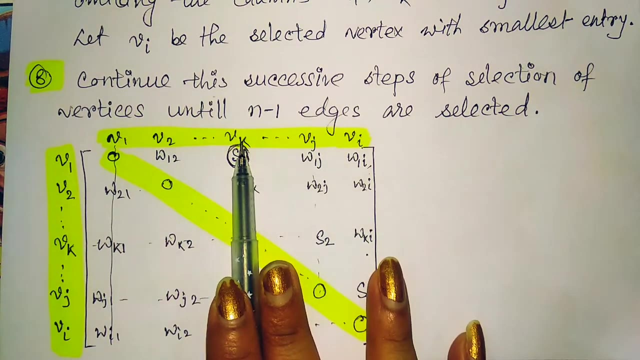 So, once a vertex has been selected, corresponding to that particular vertices for The column should be omitted for the choice of minimum weight. So V1 and Vk among these two. After Omitting these two column entries from the remaining options. 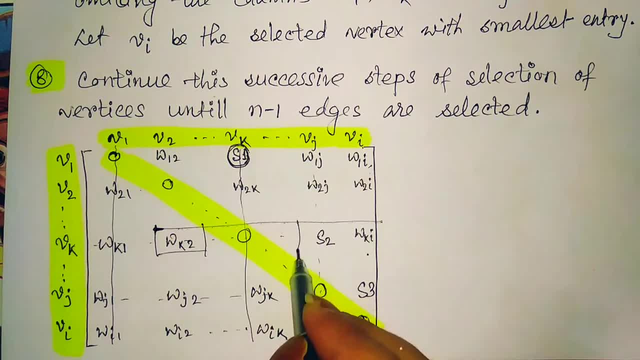 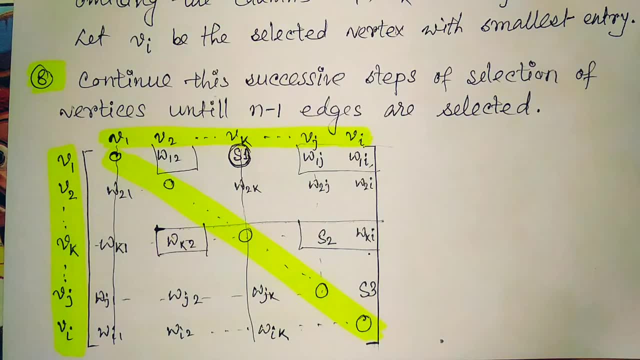 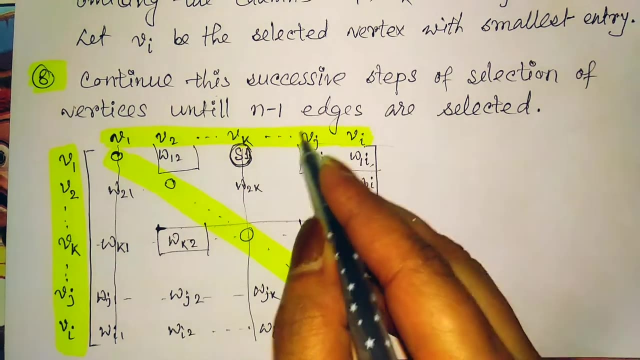 That means remaining option is this: are Here this one and this one, and this one and this one? From this options we should search that which one is the minimum weight value Corresponding to that minimum weight value. we should decide: Let Vj is the minimum weight value. we will find out. 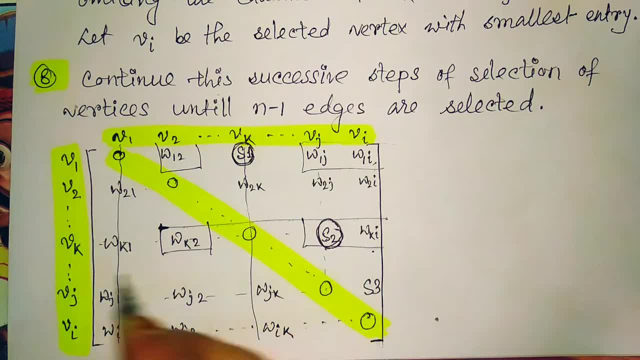 So we should select this one. So the next vertex chosen Is Vk, Vj, So that is the age which we should choose in the spanning tree. So, after choosing of this one, In the next step, what we will do. 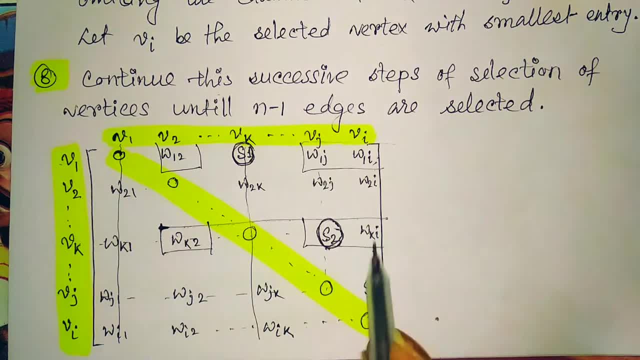 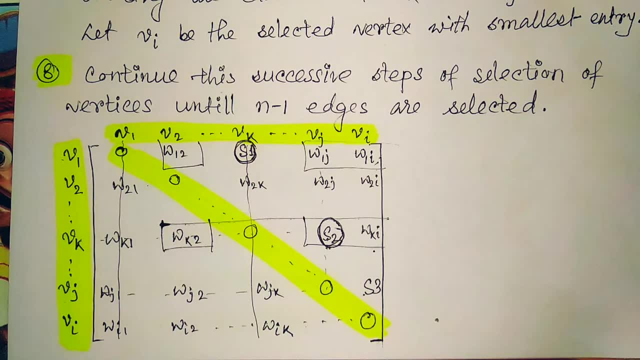 We consider the column V1,, Vk and Vj. Remember which row we have taken previously. While we choose one vertex as the entry vertex, We should include one extra row Corresponding To that chosen vertex, But we should not leave the previous rows even. 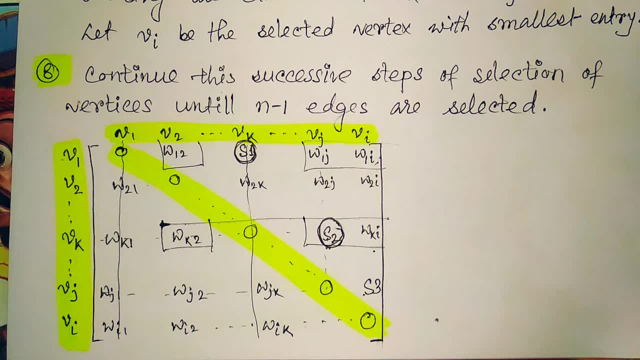 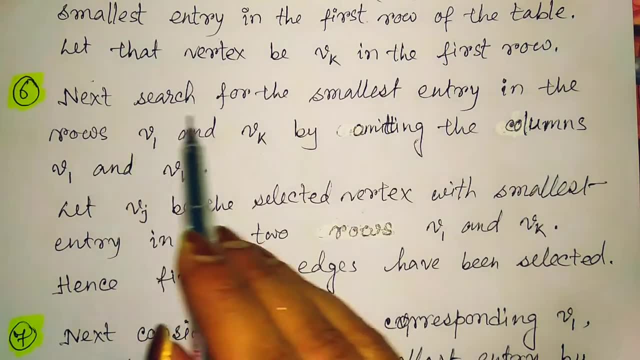 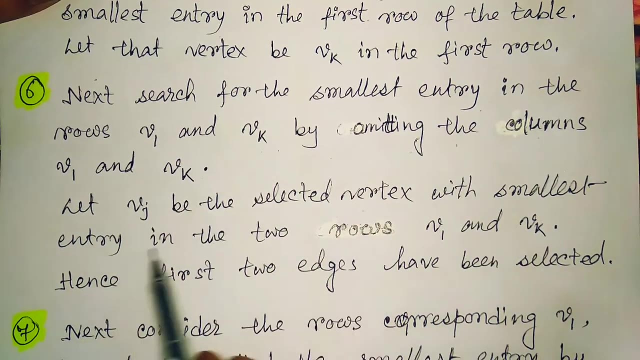 What we will do. We just leave the corresponding columns as the rows are increases. So in the next state We search for the smallest entry in the rows V1 and Vk By omitting the columns V1 and Vk. Let Vj be the selected vertex with smallest entry in the two rows V1 and Vk. 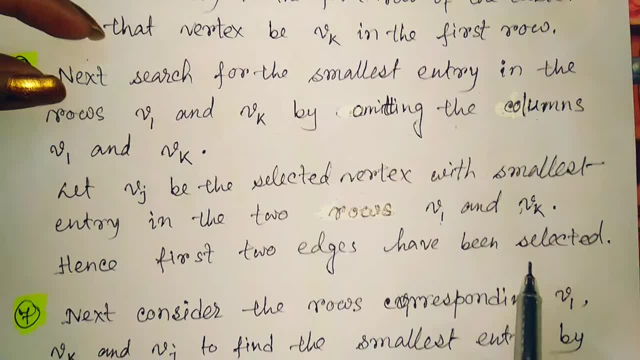 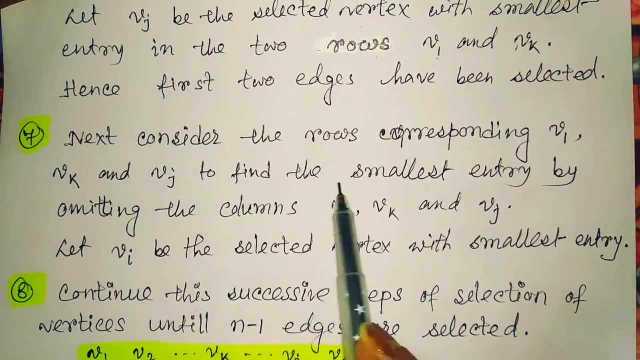 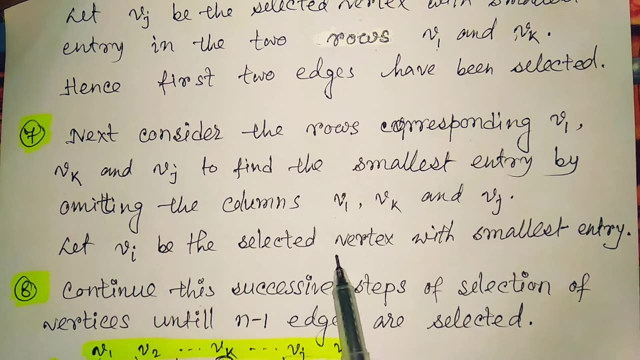 Hence the first two edges have been selected. Next, we consider the row corresponding to V1,, Vk and Vj To find out the smallest entry by omitting the columns V1, Vk and Vj. So let Vi be the selected vertex with the smallest entry. 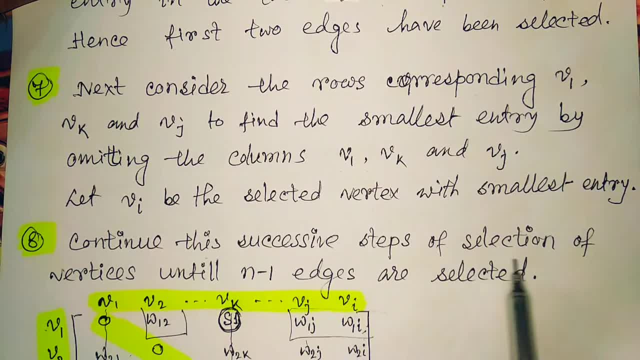 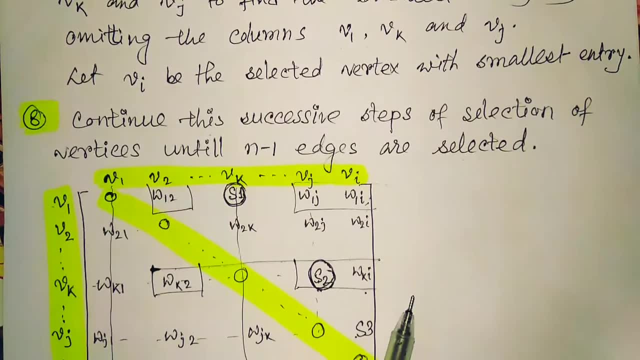 So continue this successive steps of selection of vertices Until n-1 edges are selected, Because we know If we are going to select a vertex, If we are going to create the spanning tree, In fact the minimal spanning tree, Then with n number of vertices, 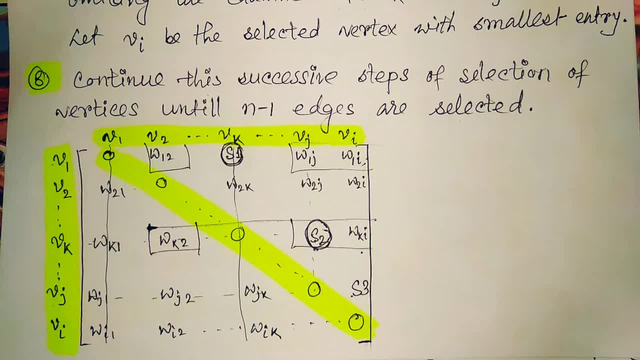 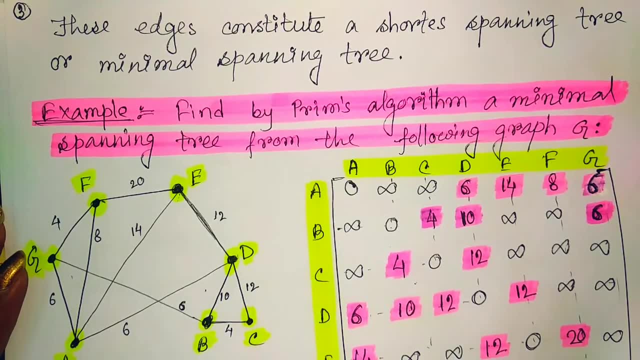 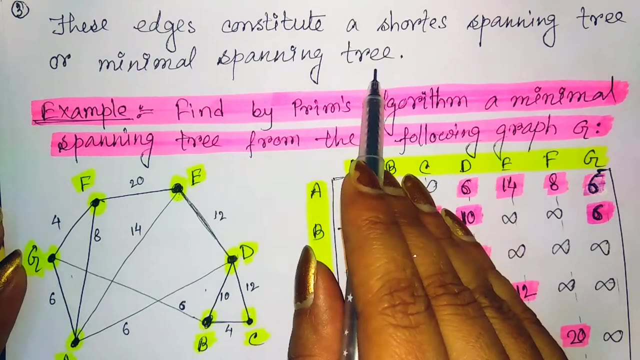 There should be n-1 number of edges. So this is the process By which we can select all the edges To require to form the minimal spanning tree. So this edges constitute a shortest spanning tree Or minimal spanning tree. Finally, we should add the weights of the selected edges. 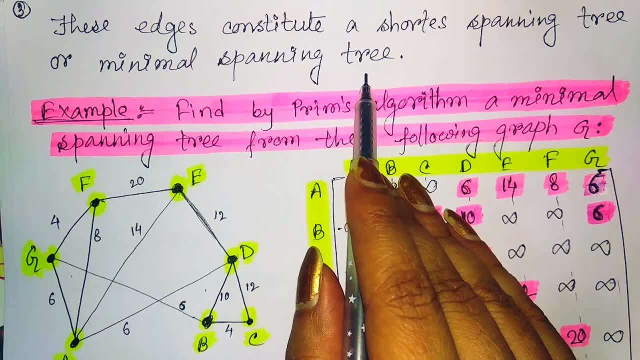 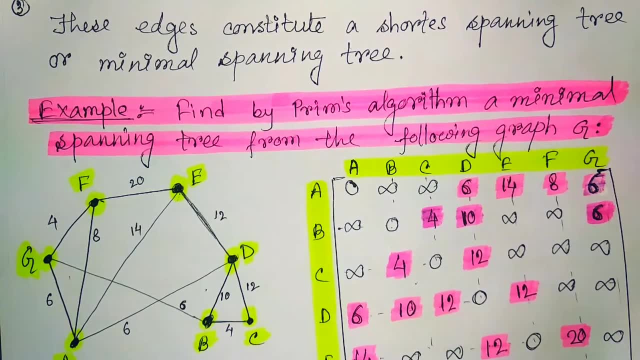 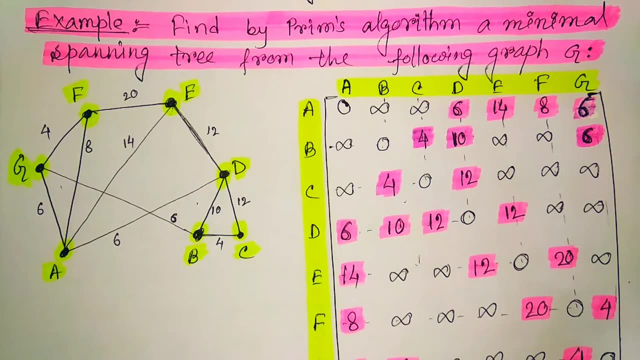 To get the final weight of the minimal spanning tree. One thing: you should remember that There may be more than one minimal spanning tree in a graph. So the entire algorithm we should discuss with an example. So what is the example Here? the find, the print. 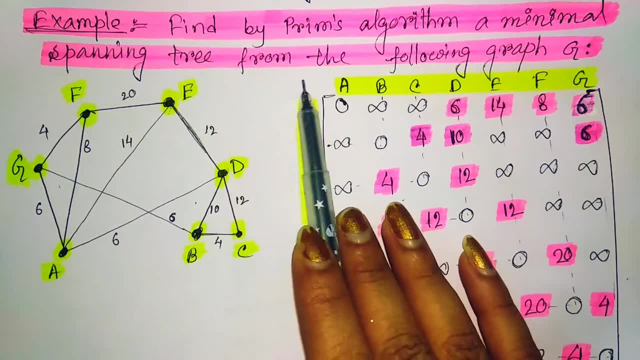 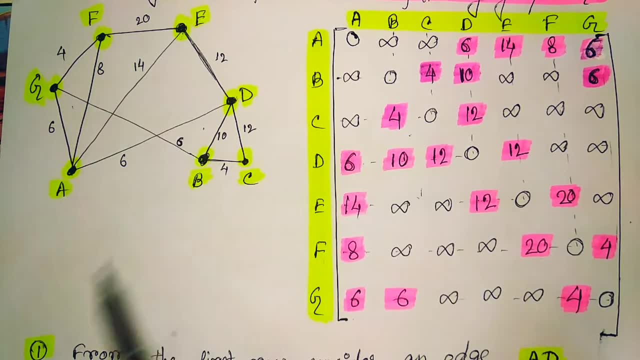 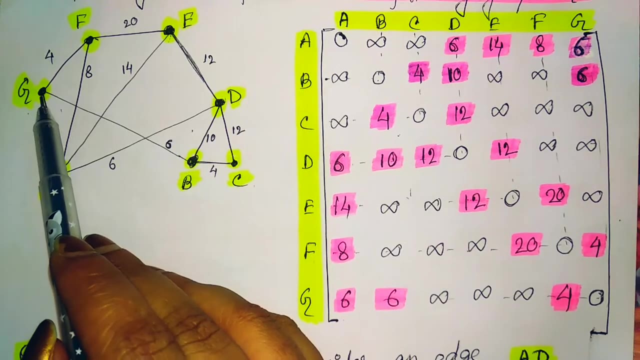 Find by the print algorithm a minimal spanning tree From the following given graph G. So the graph is given this one, And observe here The vertices are A, B, C, D, E, F and C. So total 7 vertices are given. 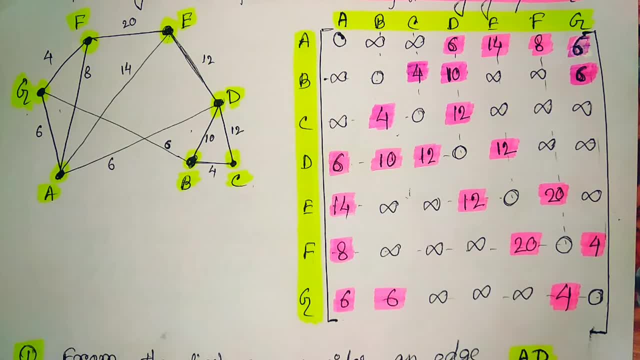 So corresponding to this vertices. and in this graph We will find out, no parallel edges and self loops are there. So this one is a simple graph. So with this simple graph, We at first create a table. The table means this is the matrix. 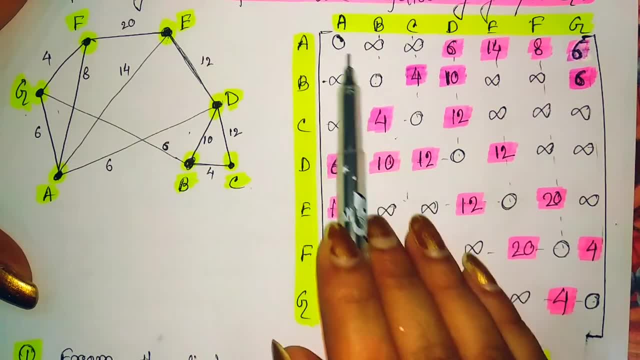 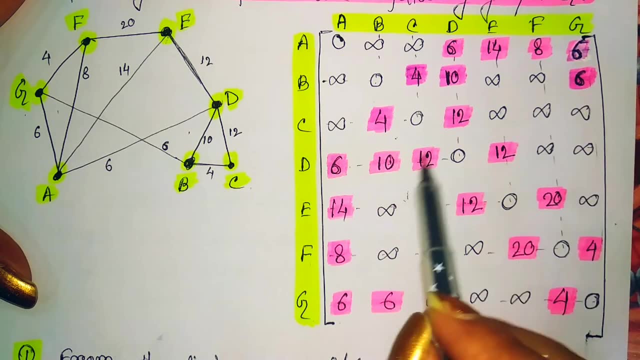 Where, row wise and column wise, we put the vertices. So here all the vertices, All 7 vertices are putted, And all the 7 vertices putted over here also Now the corresponding entry, for We know that the diagonal entries are always 0.. 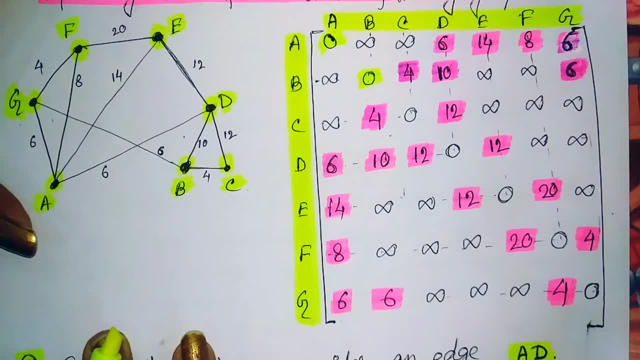 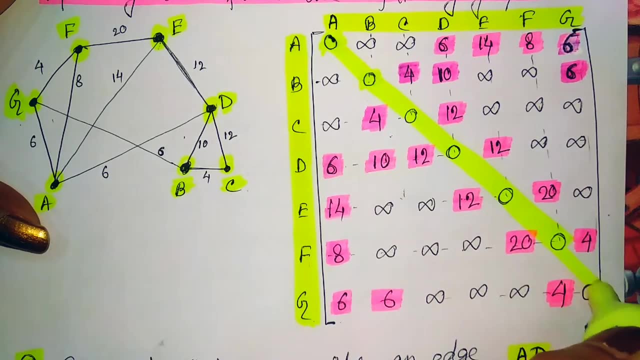 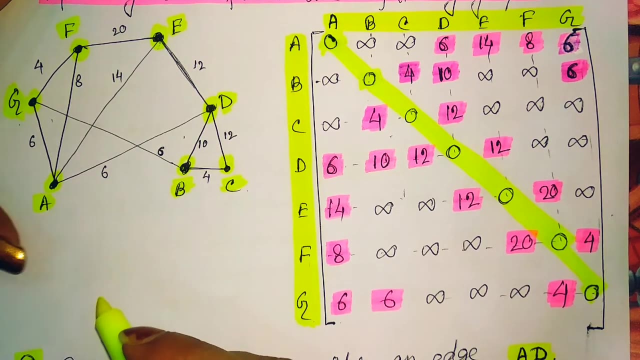 So look, all the diagonal entries are 0.. In fact, we can draw the diagonal in this way. So look, all the diagonal entries are 0.. Now, corresponding to this, Corresponding to the vertex A, We should start from one after another. 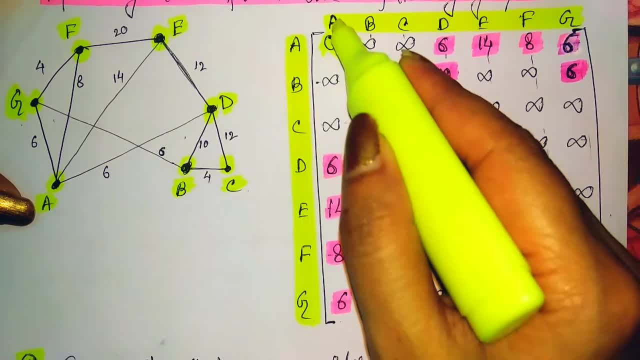 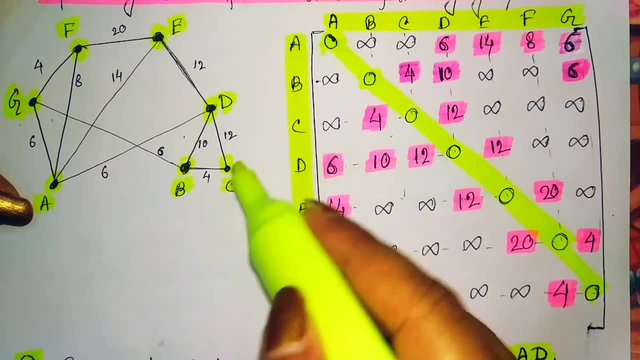 So let us start from the vertex A. So A to A, there should be the entry 0.. A to B: there is no connectivity. That's why it has to be infinity. Then A to C: again no connectivity. So it should be infinity. 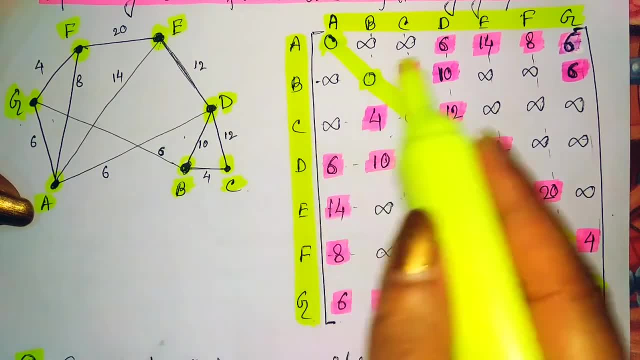 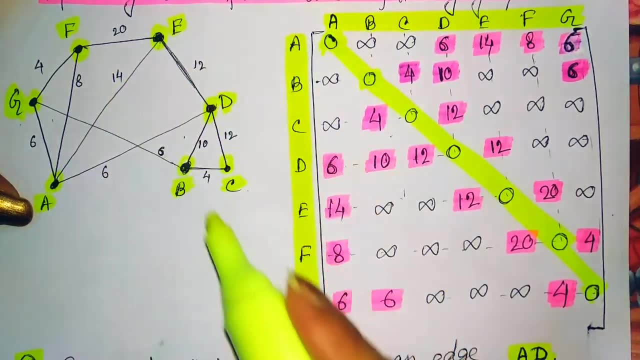 Then A to D: there is a connection And its value is 6.. That's why this is the 6.. A to E, its value is 14.. Then A to F, its value is 8. And A to G, its value is 6.. 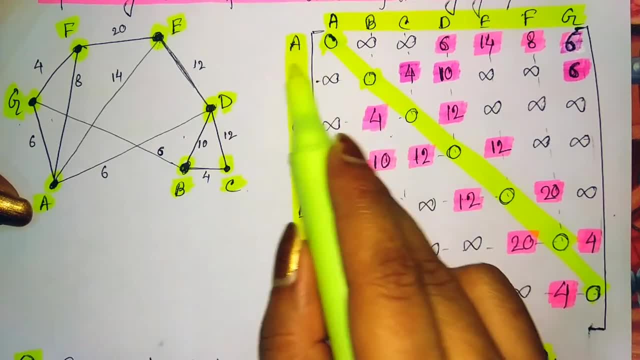 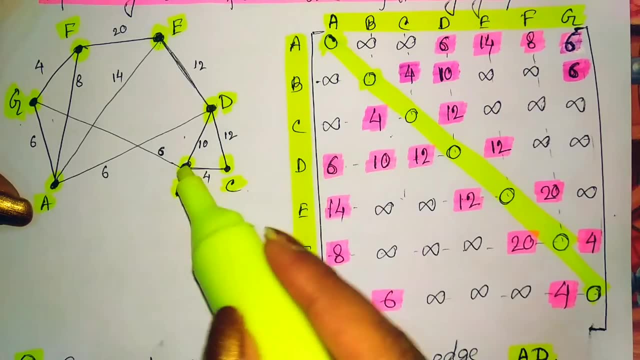 So from A, what are the connectivities For all other vertices that we have recorded? Now come to the vertex B. So from B to A there is no connectivity, So it should be infinity. B to C, it is 4.. 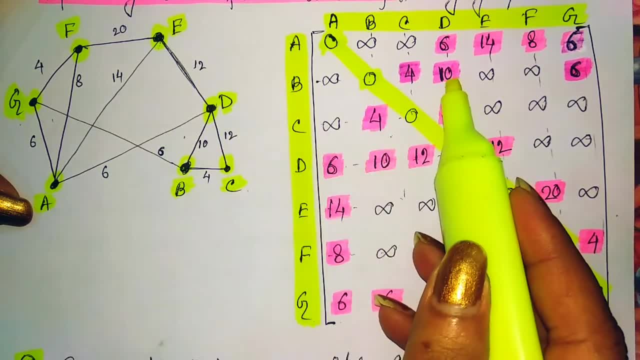 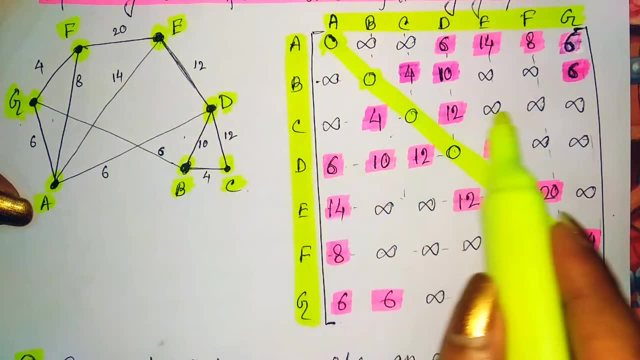 B to B: definitely 0. Then B to D, it is 10.. Then B to E: no connectivity, So it is infinity. B to F: again no connectivity, So infinity B to G, it is connected And the weight value is 6.. 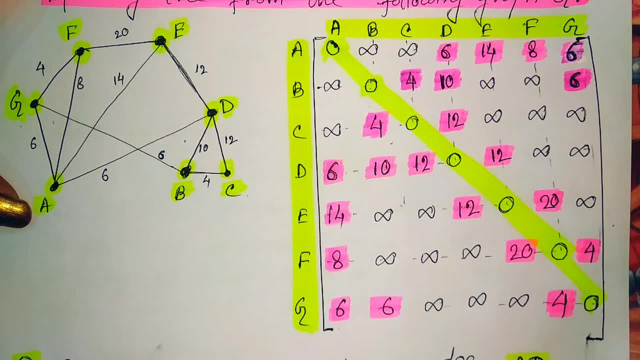 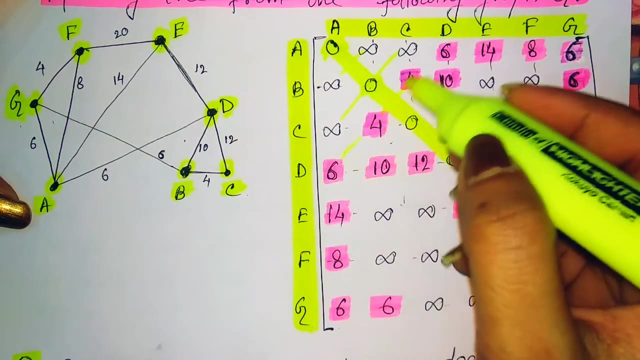 So it is 6.. Likewise, we just put all those entries And just observe this matrix carefully, You will find out this one is a symmetric matrix. Just observe if this one is the diagonal, Then you just find out that this one is the symmetric matrix. 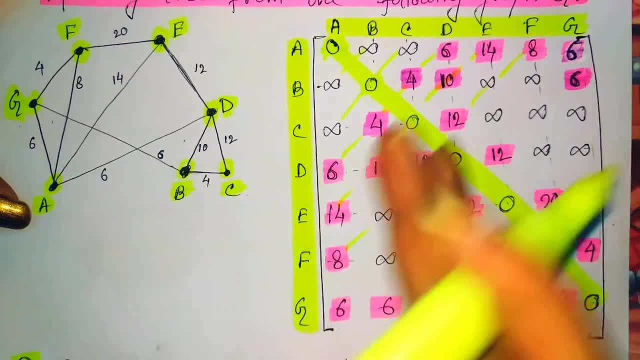 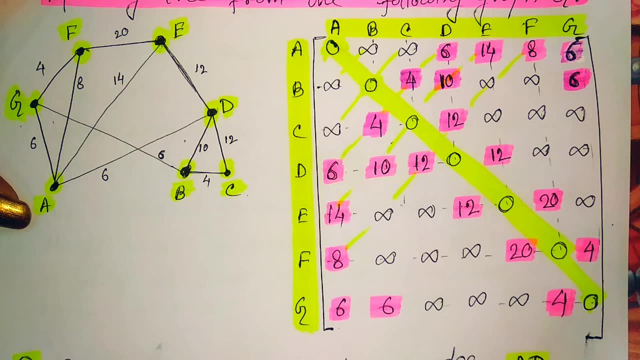 Just look, if we think this one is the mirror, Then we just find out the mirror image of this one. So this is the table which we should form by the given graph. After forming formation of this one, Now we should find out the spanning tree from here. 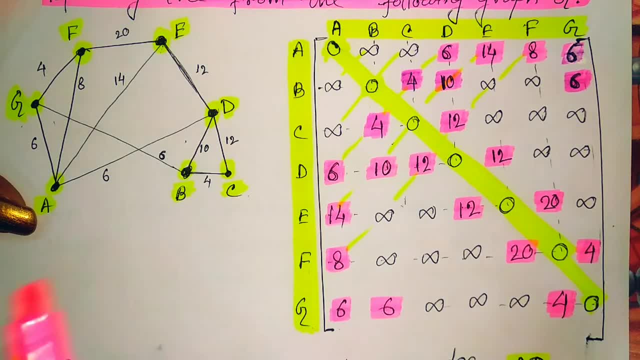 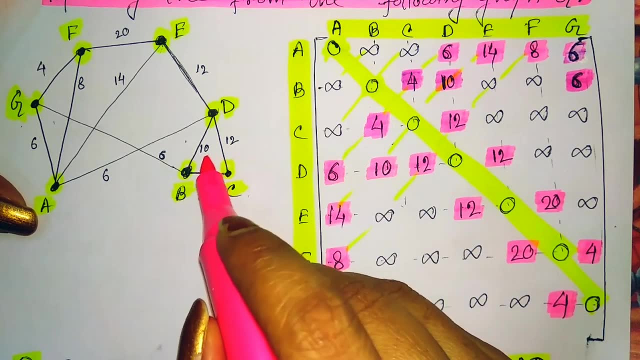 So what we will do, we should start from the first row, That is, the row A. So in this row A at first, we find out what is the minimum Entry, What is the minimum entry. So minimum entry is here 6.. 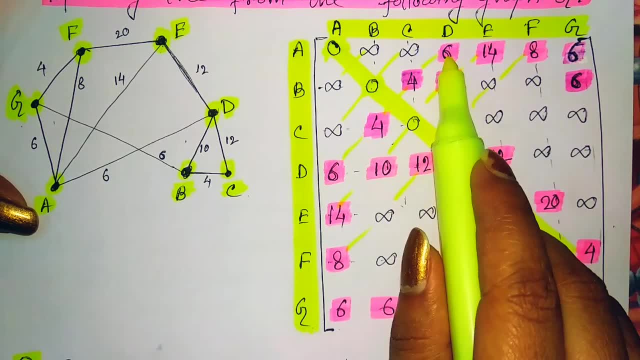 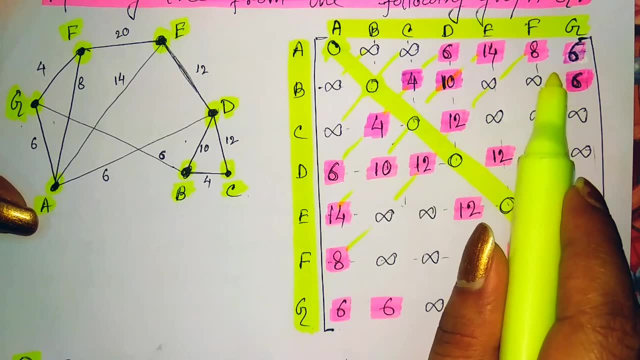 But 6. we will find out at two places, At the place D as well as G. If you will have such a tie, Then you may choose any one of these two. So initially let us choose. the first chosen vertex is D. 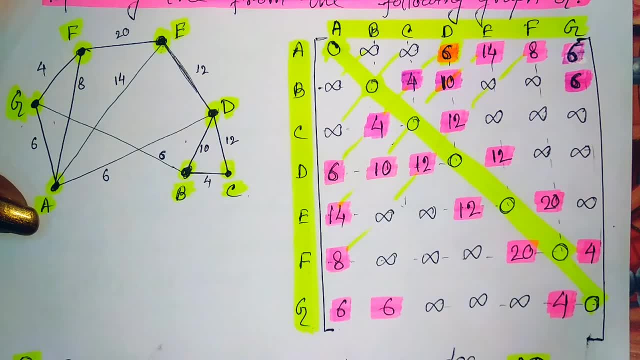 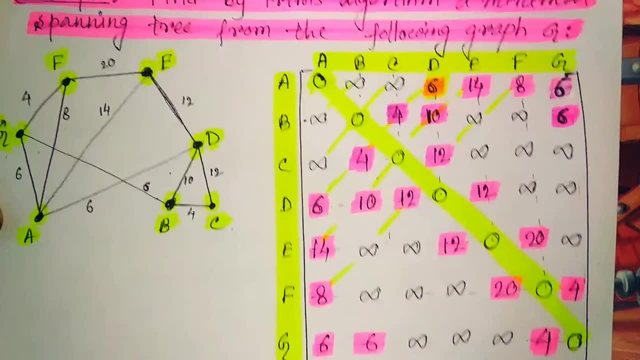 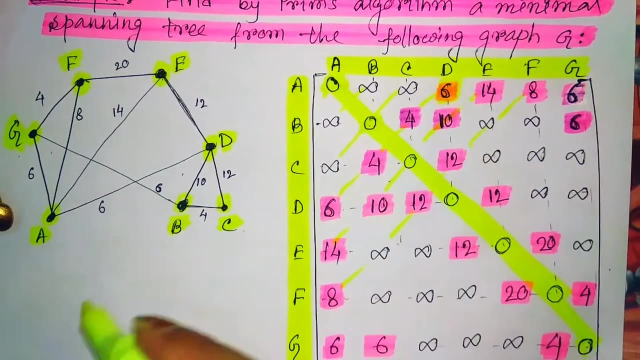 Any one we may choose, and we choose it is as 6.. So that here from the first row, consider an edge AD. So look, we should consider AD, Because this is the entry AD. So we have taken here the AD. 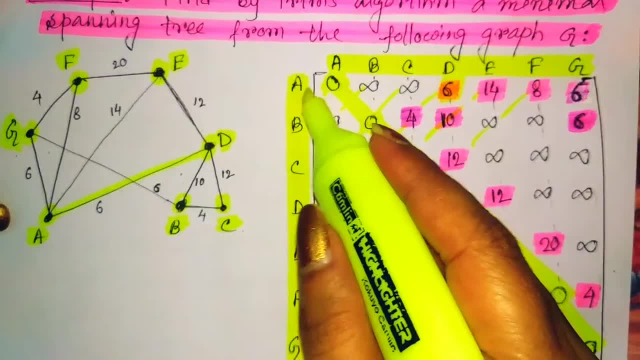 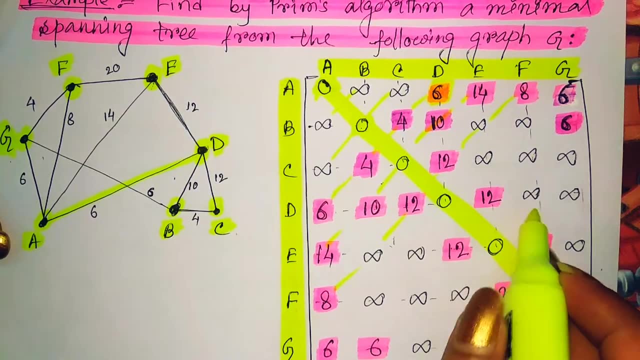 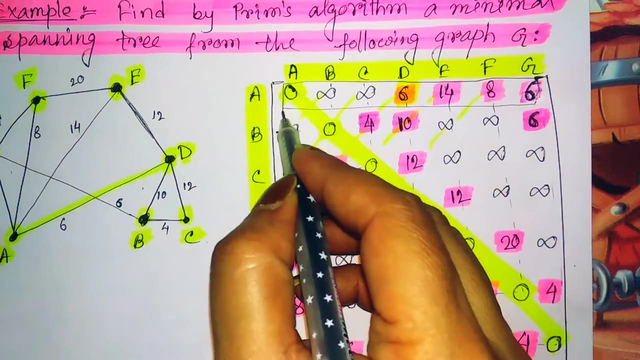 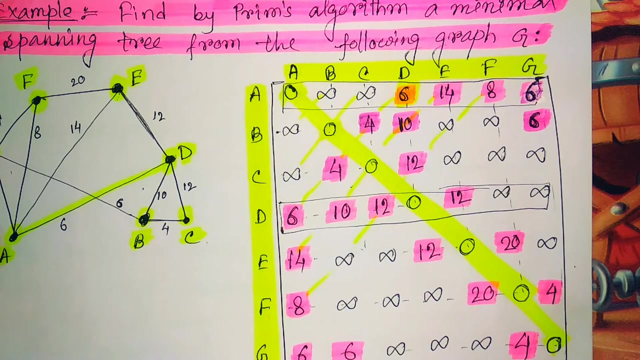 Now the row A and row D we should consider for the next. So row A means this one, Row A is this one And row D means this one. Among these two, we should omit the first row, First column, sorry, And the D column. 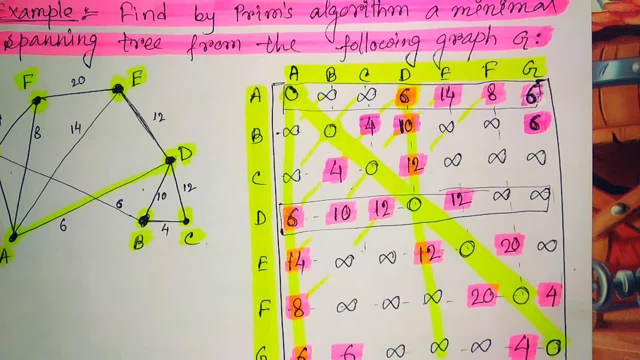 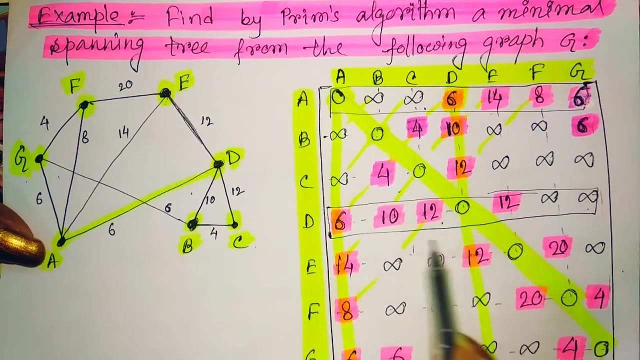 Because we already have chosen these two vertices. So now, from the remaining Remaining means, the entries are these two Here: this 3 and this 2 and this 3.. Among these entries, which one is the minimum value? So the minimum value here we will find out that it is 6 only. 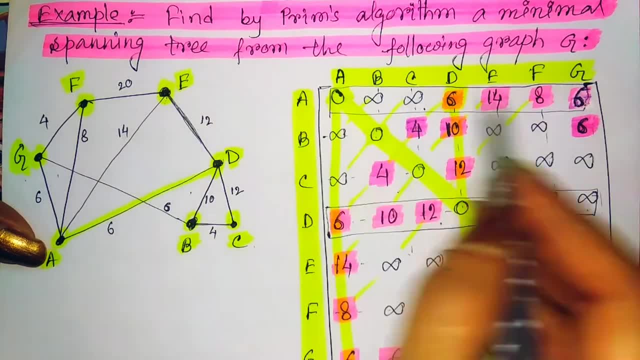 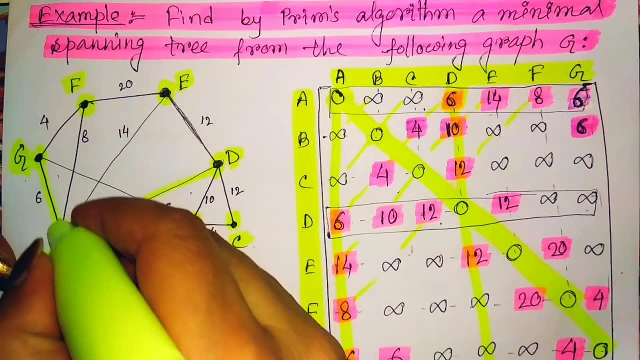 So 6 means this position for AG is the next choice of the edge Which we should select in the spanning tree. So AG is the next choice for the selection, So that we should write down here from the row A and D: 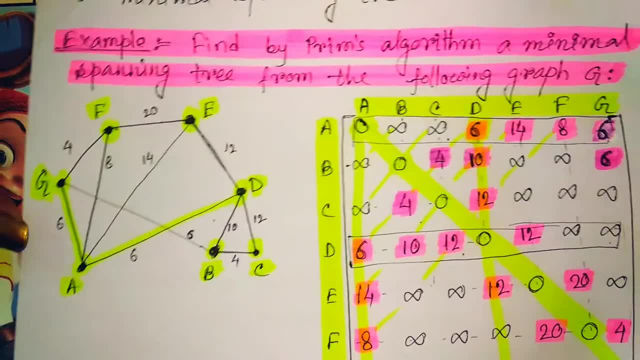 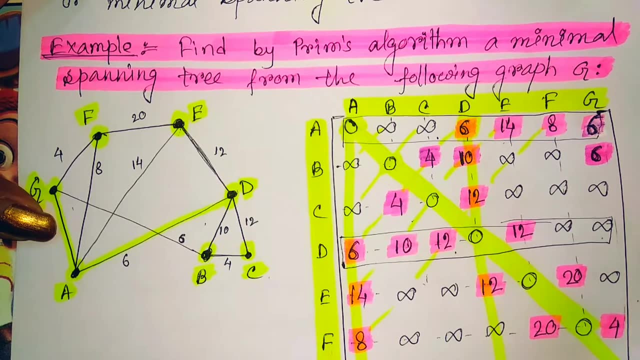 Select the edge AG. Now what we will do. We will have now 3 rows for our choice. One is A, Second one is D And one another one is the G. So G means this one. So here G we have taken. 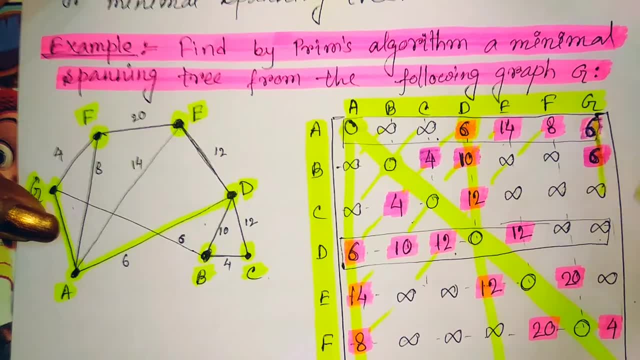 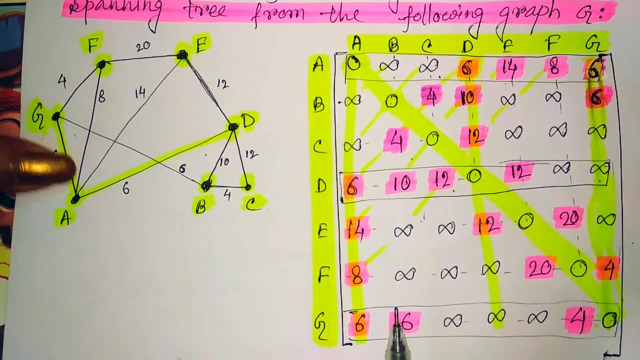 And we should omit this column, Because this column we should not consider now. So, omitting these 3 columns and considering these 3 rows, What we will find out here? We will find out that the minimum entry corresponding to here it is 4.. 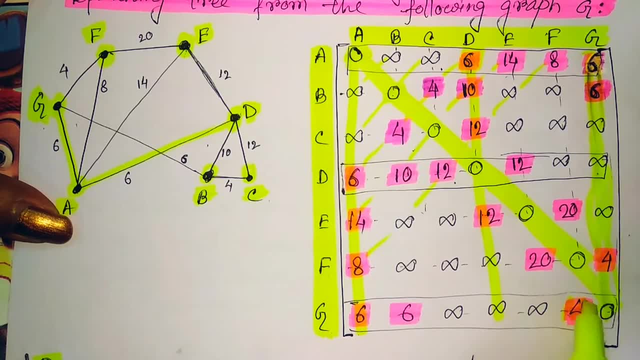 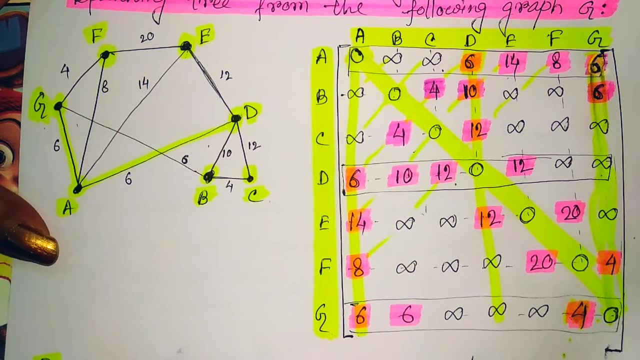 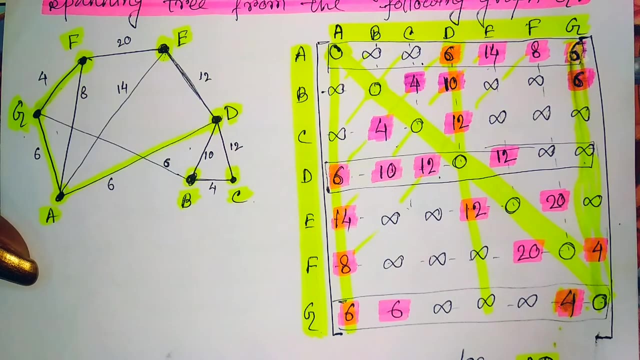 So the minimum entry we will find out here it is 4.. So 4, this position is the GF, So that we include next the edge GF means this one, Next we include this edge GF. So in the next consideration we consider this one, this row also. 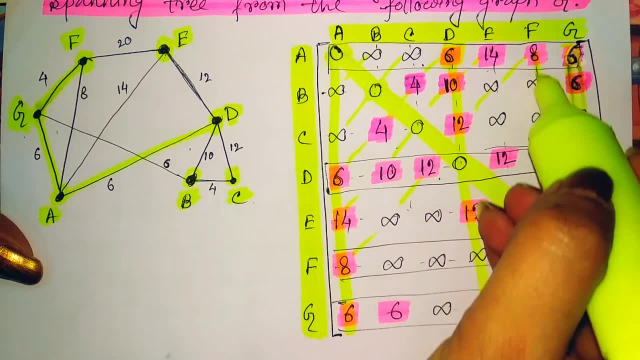 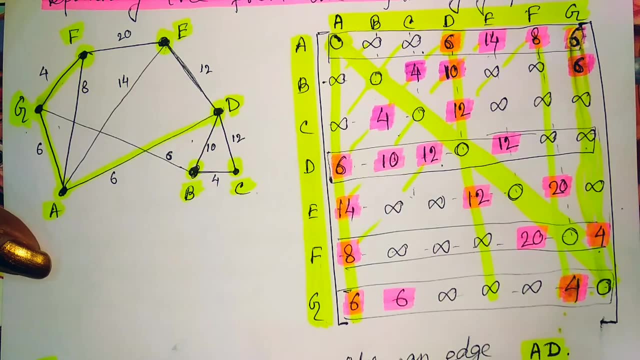 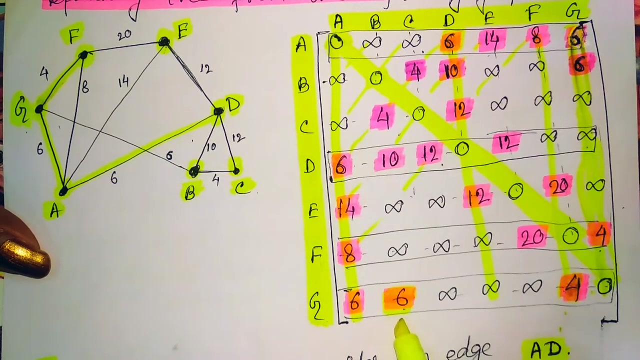 And we definitely Remove the edge column corresponding to the vertex F. So, after this removal from the remaining portions, What is the minimum entry? The minimum entry is now, it is 6.. So this one is our minimum entry. So this position is GB. 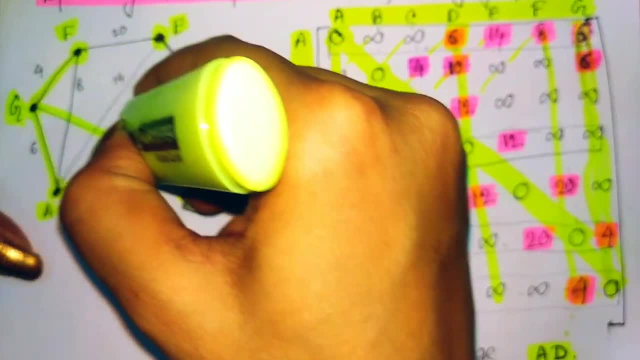 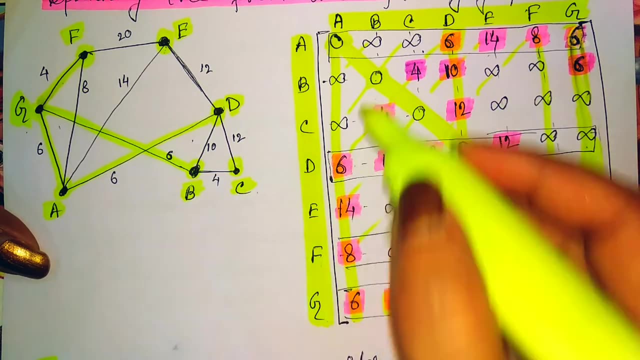 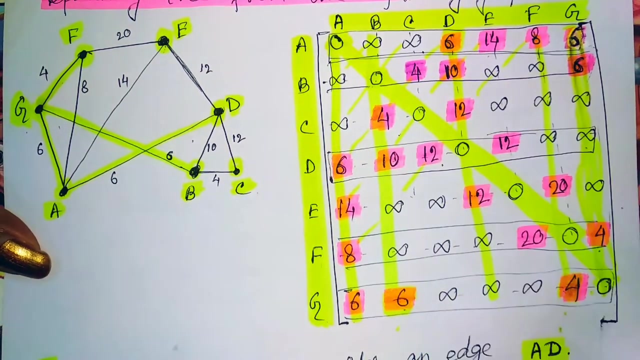 So next we include the edge GB in your spanning tree So that after that the B is selected and B column should be omitted. So B is included and B column is omitted. Now from the remaining portions, what is the minimum value? 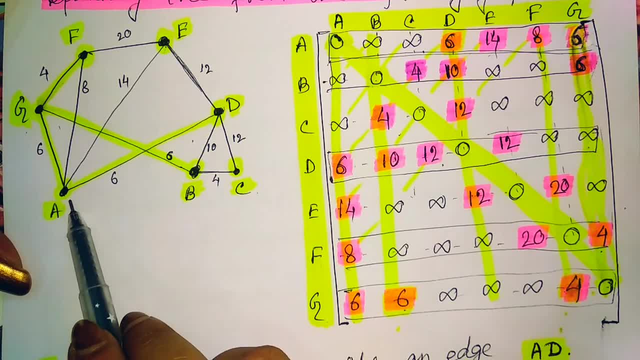 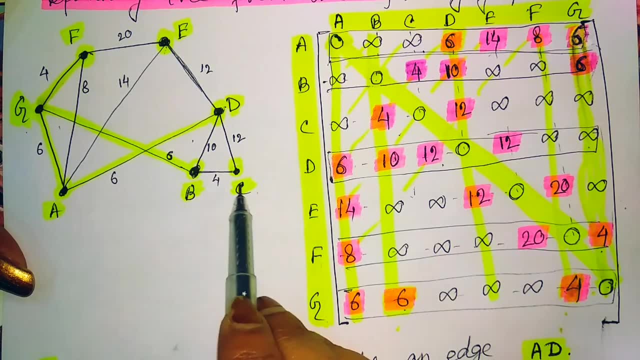 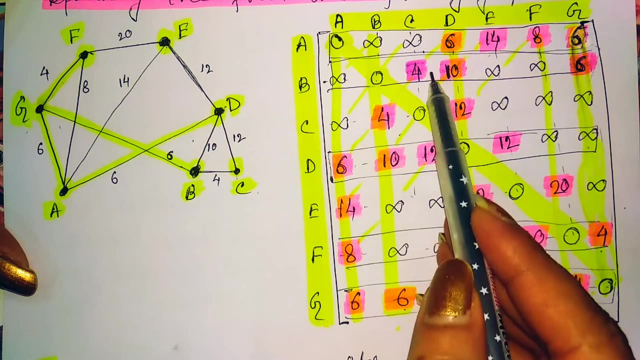 So at first we just observe here that A, D, then G, F and B, All those vertices already selected, Our remaining is C and E, So that we should emphasize on the column C and E only, So here in the selected rows, we will find out that this one is the minimum entry. 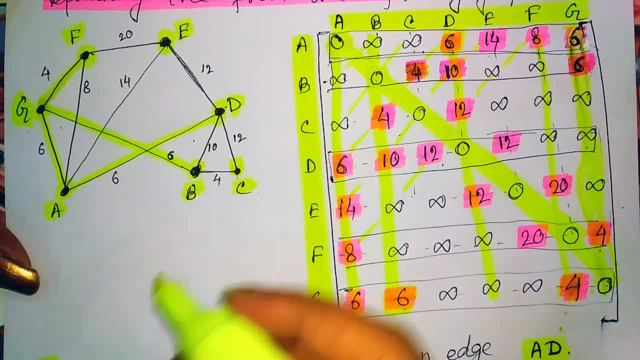 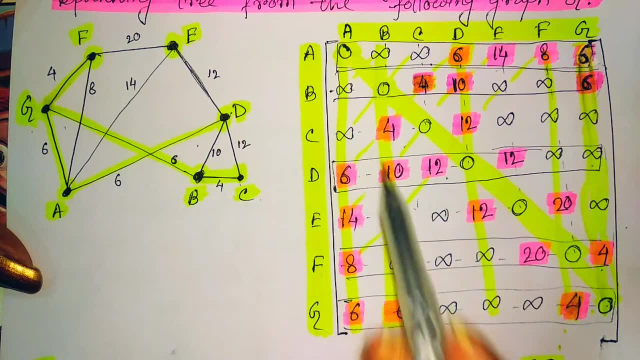 This one is the minimum entry, So that is the position BC, So that we consider this edge BC in the spanning tree. So after doing this one, we consider this one also for our choice of selection And we omit this column again. 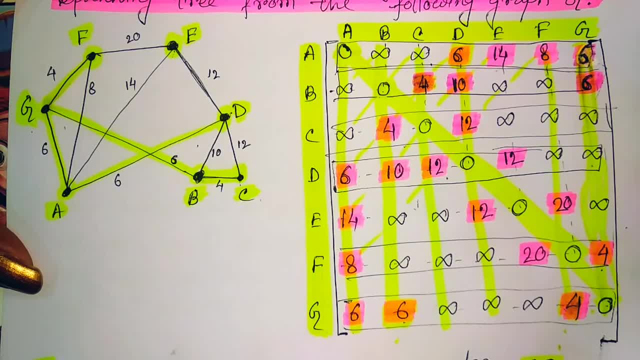 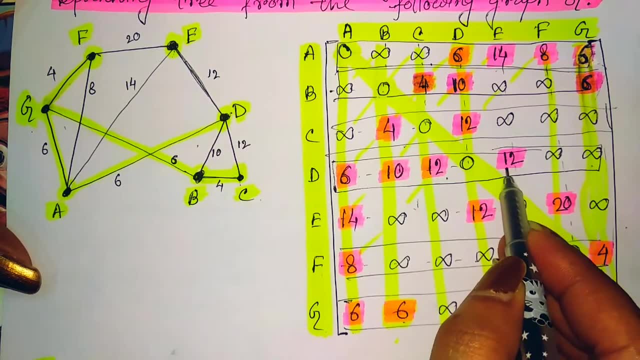 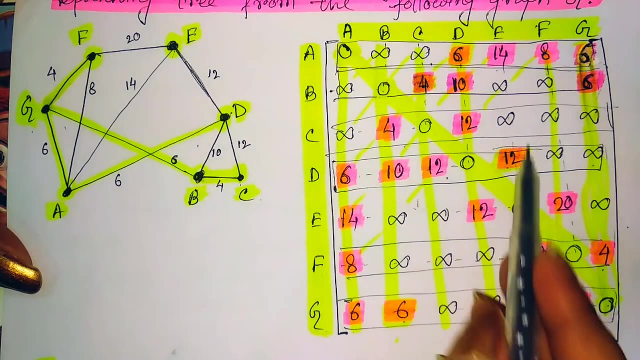 So now the remaining column from where we should find out the next minimum, is the only E, because only the vertex E is left. So here the minimum entry is the 12. So this corresponding, we will find out the next edge. So this position is DE. 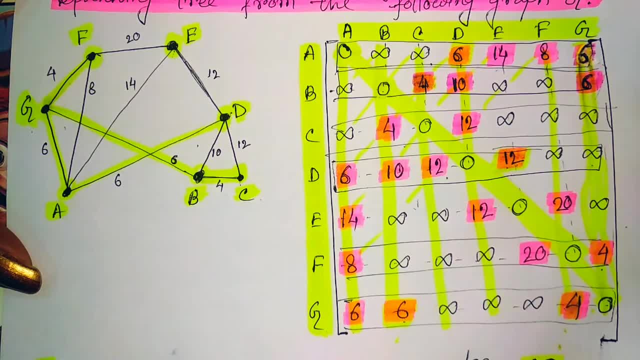 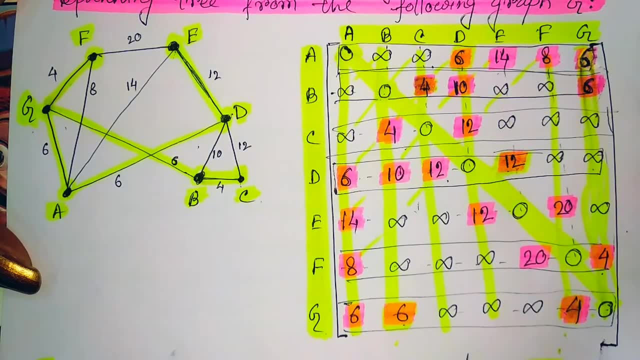 So we should include next the edge DE. So this one is our next edge in the spanning tree. So after doing this one, We will selected all those vertices, That means all those rows from we have the entry. So for all vertices we have the entry. 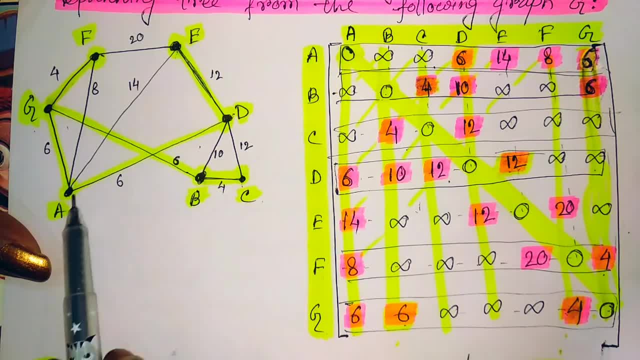 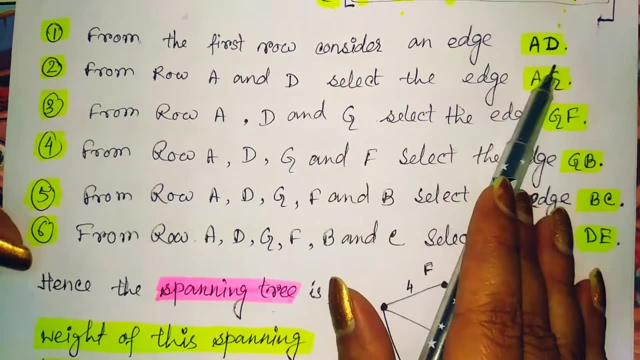 So finally we get our spanning tree And here all the yellow lines constructing the spanning tree. So just look the summation here. So from the first row we consider AD. From the second row that means not second In the second step, from row A and D. 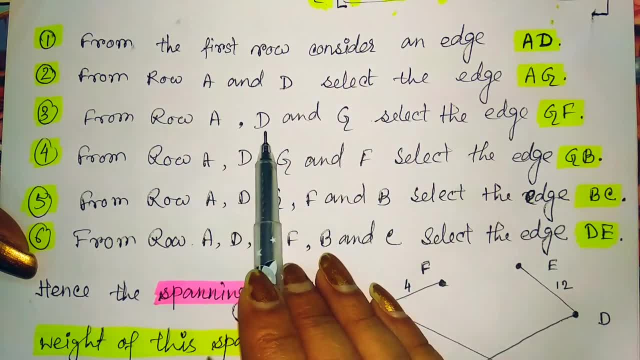 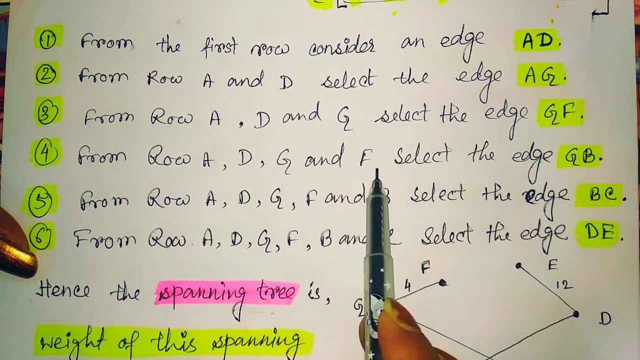 We select the edge AG. From the row AD and D, AD and G, We select the row GF. From the row AD, G and F Select the edge GB. And from the row AD, G, F, B, We select the edge BC. 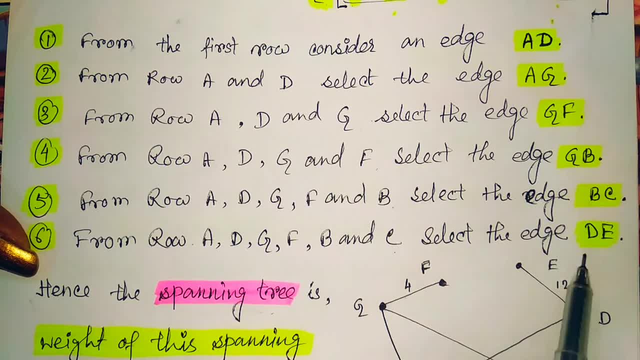 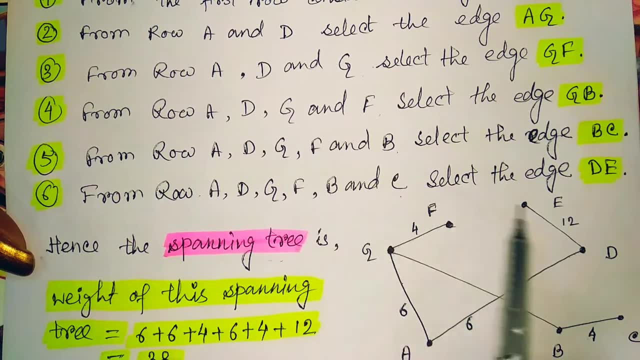 And from the row AD, G, F, B and C We select the row DE. So by considering this one We finally create our minimal spanning tree like this way, And the minimum weight is 6 plus 6 plus of here 4, then plus 6, then plus 4 and plus 12.. 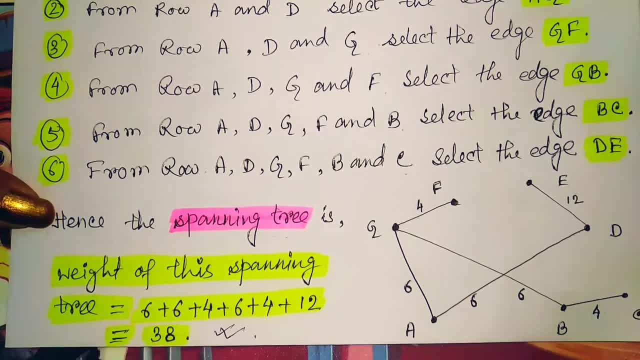 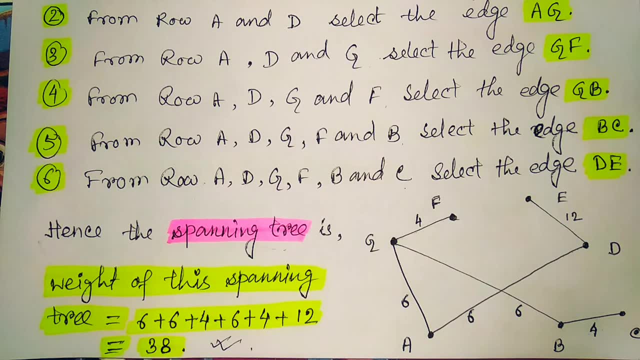 So finally it is. the 38 is the minimum weight value for the given graph, From where we will find out the minimal spanning tree. So this is our PRINCE algorithm to find out the minimal spanning tree. Hope it is not that much difficult. 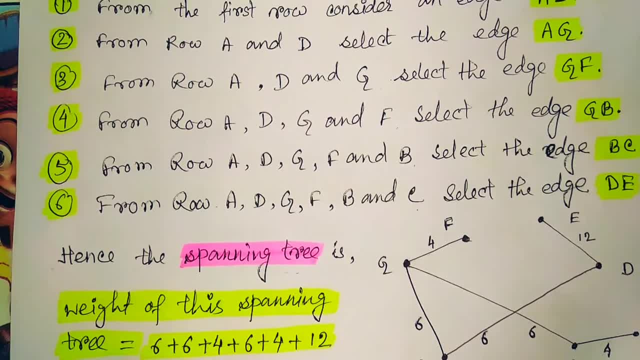 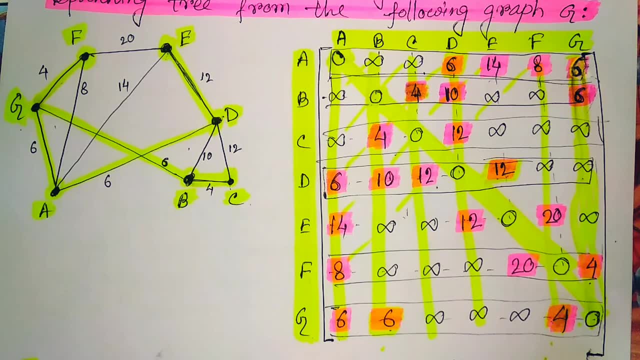 Just go through the video once again To understand the entire process, Step by step evaluation is given here. I hope you understand. Thank you all. Have a nice day.